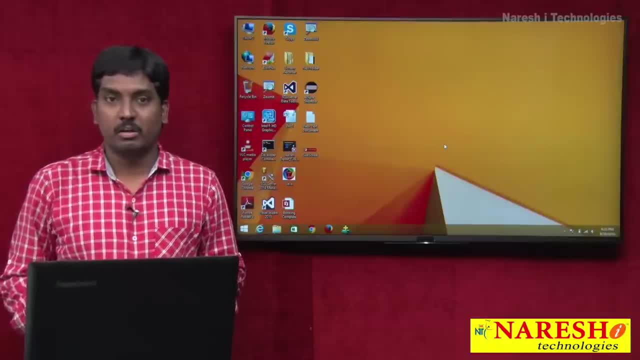 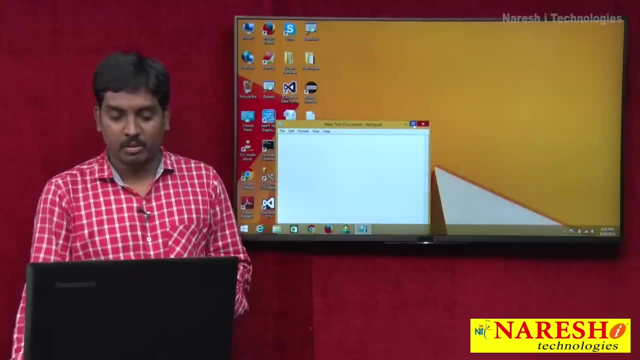 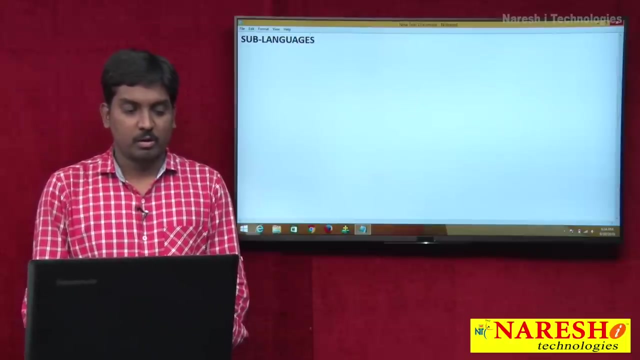 and later we will discuss one by one query syntaxes. And now I just go to here the first. we will see the sub-languages of SQL. So what we called here sub-languages, Sub-languages, Okay, Languages, Okay. So sub-languages of SQL, Okay. So now we will discuss here the 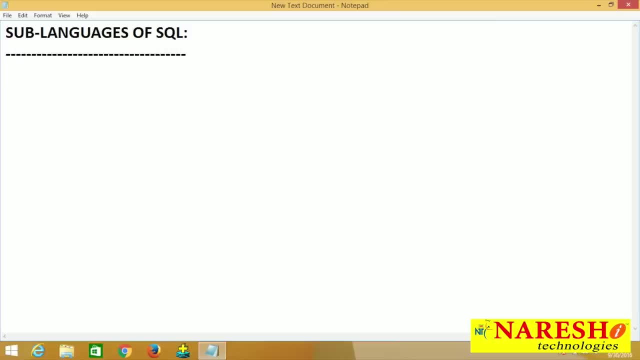 total sub-languages of SQL language. Now we will discuss now here. observe the first language we called here. my first sub-language of SQL is called as a DDL. we called Okay, So it is called a data definition language. Okay, So first one data definition language and 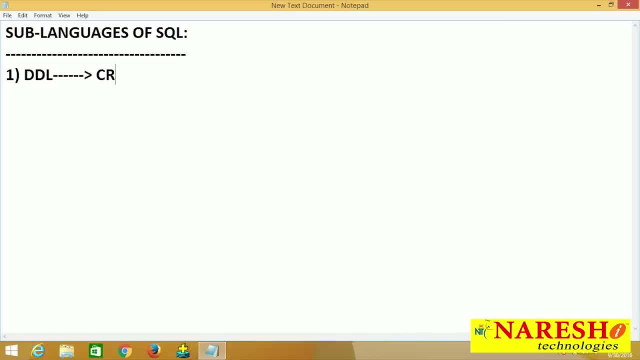 this language was having here The sub-languages are there. Okay, In that first command is create. Okay, So create, and later have your alter. And later I have here the SP underscore read name. And the next one we are going to use here truncate. Okay, We are using here truncate and finally drop. 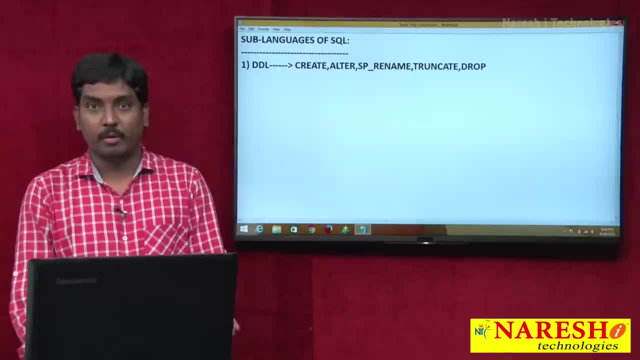 commands: Okay, So these are what it is here. DDL commands. we called: Okay, So there are five commands. was there in this language? DDL language. Okay, So here it is. So our sub-languages are there. Okay, So here it is. there was five commands. 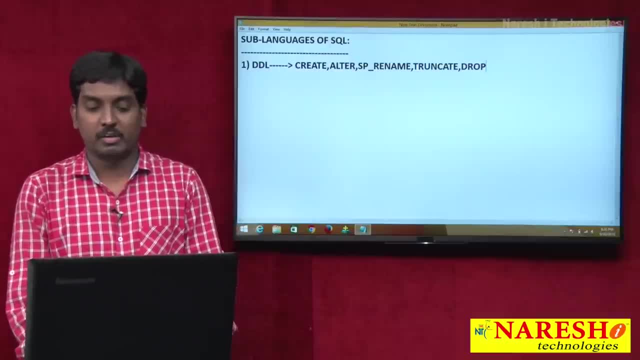 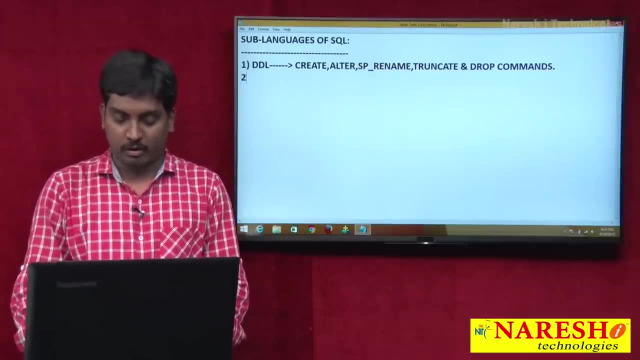 Okay, So I have here sub-languages, sub-languages there. sub-languages are there, sub-languages have. So those are: create, alter, SP, underscore, rename, truncate and drop. And next one, the next sub language of SQL that we called as a DML language. DML is nothing. 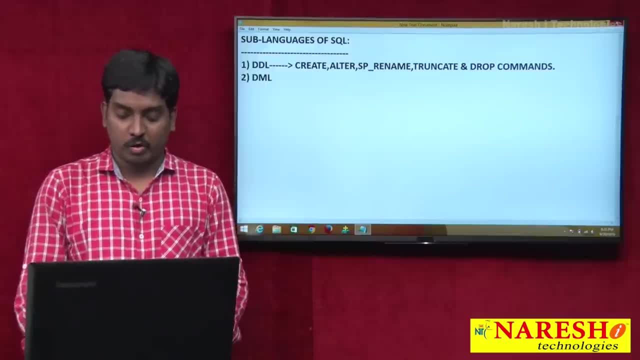 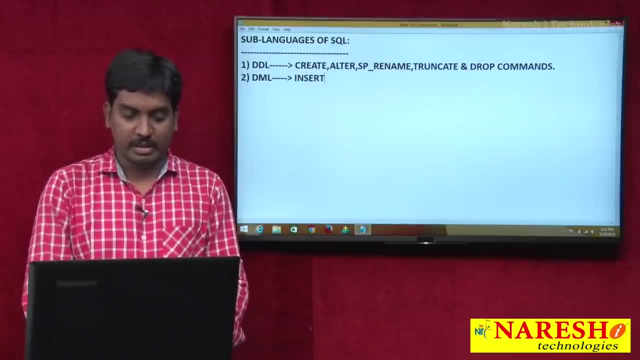 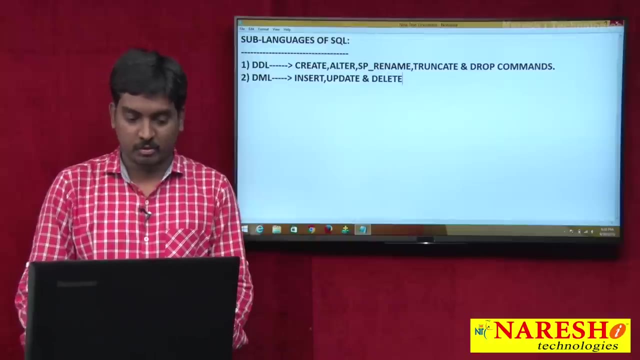 but data manipulation language. So in this language we have again. some queries are there here that we called here. first one, what we said, insert and update and finally delete commands. So these are comes under your DML language. And the next one, next language we called here DQL, is nothing but data query language. 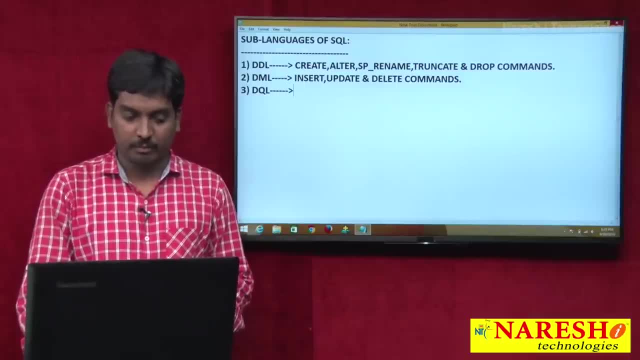 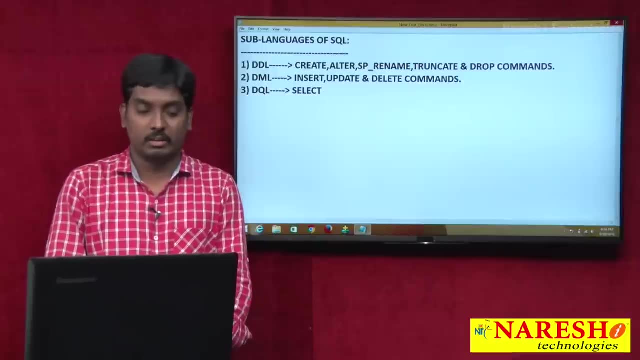 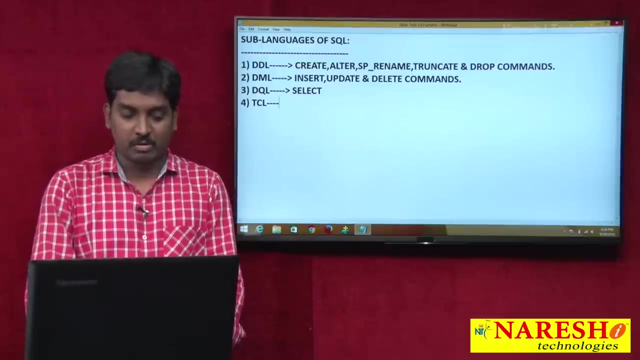 So in this language we having here, in this language we having now, so the only one command was there. in the language The command is called as a select And later the next language we called as a TCL is nothing but transaction is nothing. 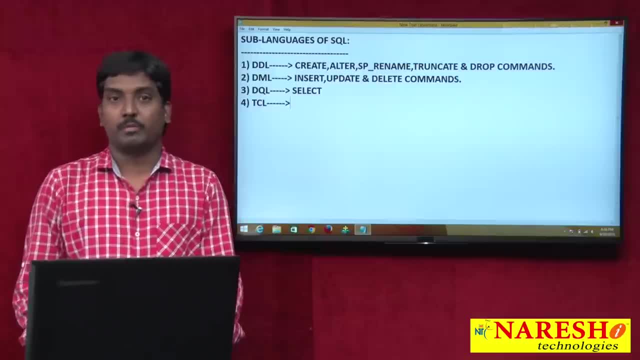 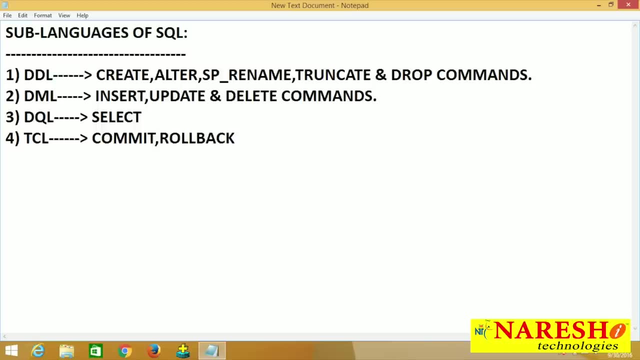 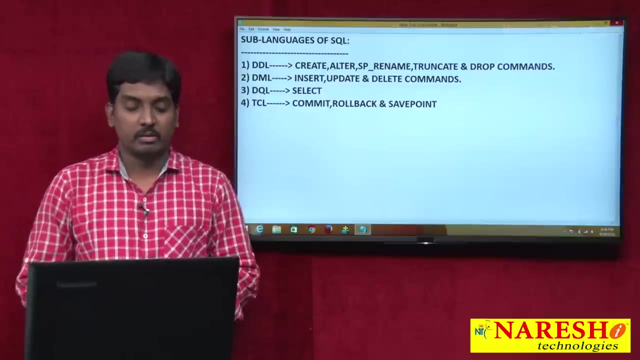 but transaction control language we called. This language was having here commit and the second one we called as a rollback And the third one we called as a save point. So in this language, commit, rollback and save point, which will comes under DML. 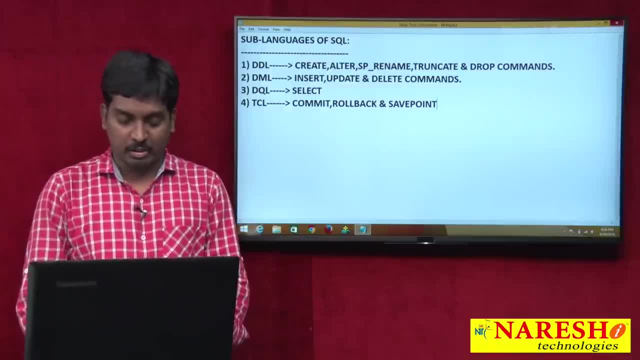 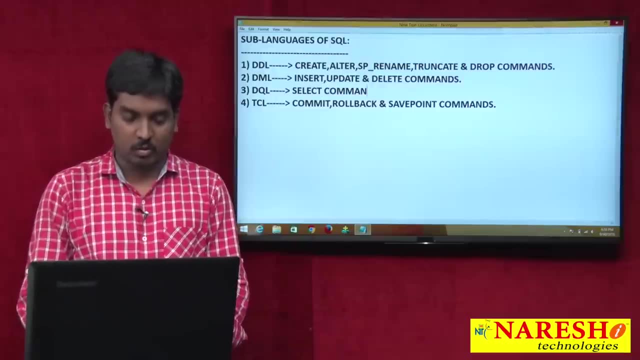 Transaction control language. So these are transaction control language commands. I can say, now And here the TQL was having only one command, that is called a SQL command, And later we have the final language and the final sub language we called. that is called: 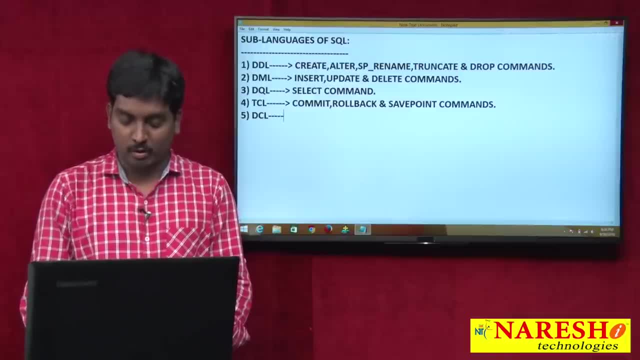 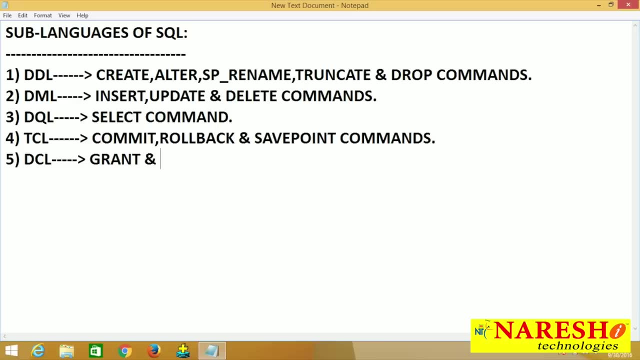 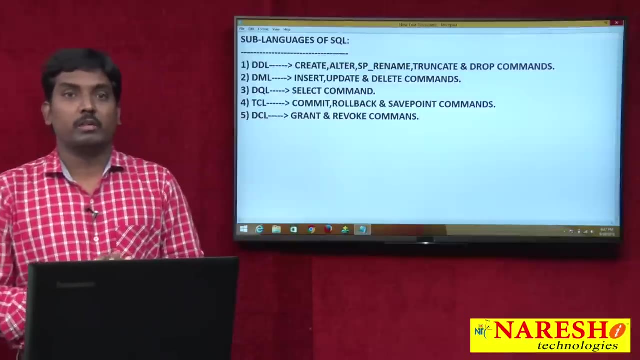 a DCL is nothing but data control language. So this data control language was having the two commands here. one is called a grant and revoke. Okay, So revoke commands. So these are what it is here. The total five sub languages of SQL structure. query language: okay. 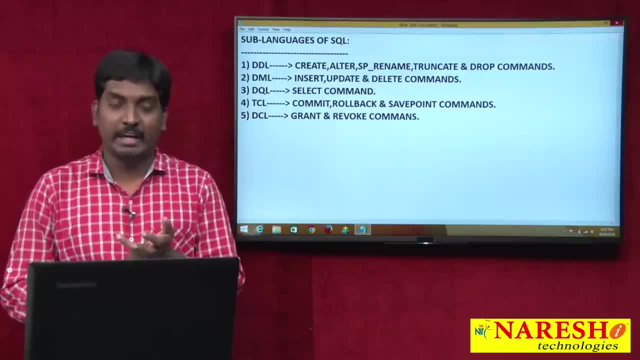 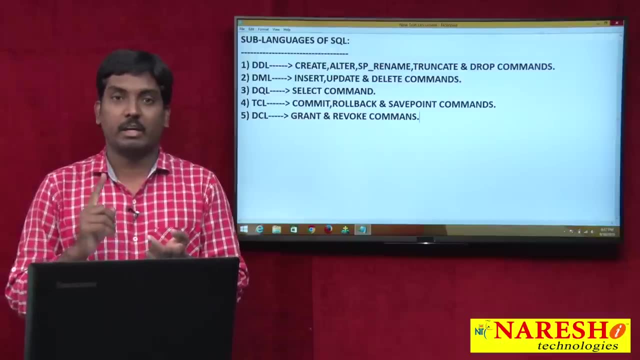 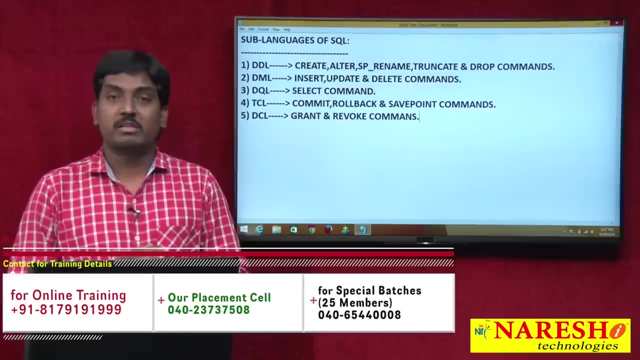 So that means each and every language, whatever we discuss here- DDL, data manipulation- okay, what we can say? data definition language, data manipulation language, data query language, transaction control language and data controlling language. So these are the five sub languages. was there? 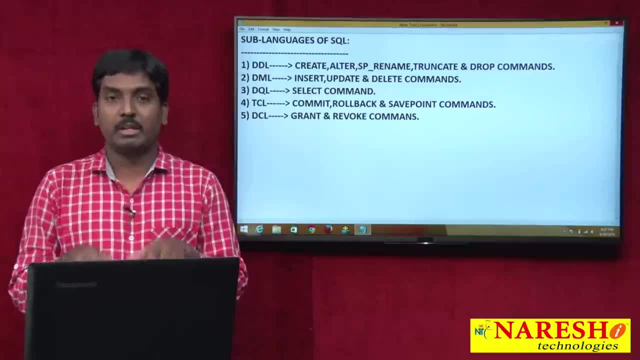 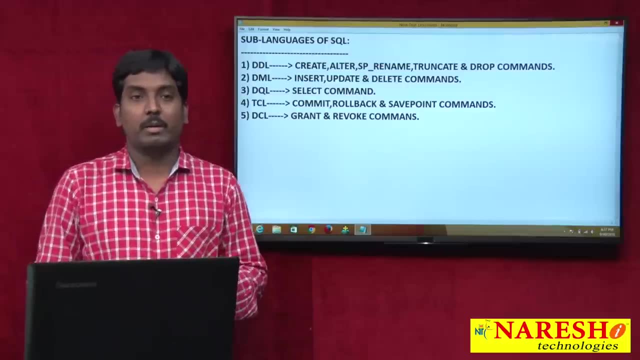 In SQL, But every language was having some specific commands and those commands we are going to use them to perform your database operations. okay, So let us see that all commands. okay, we will go to see one by one. okay, how to write. 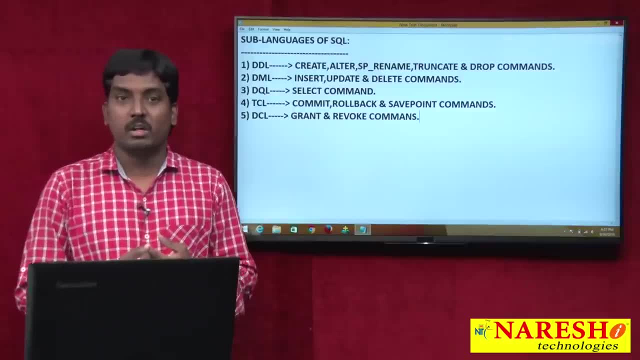 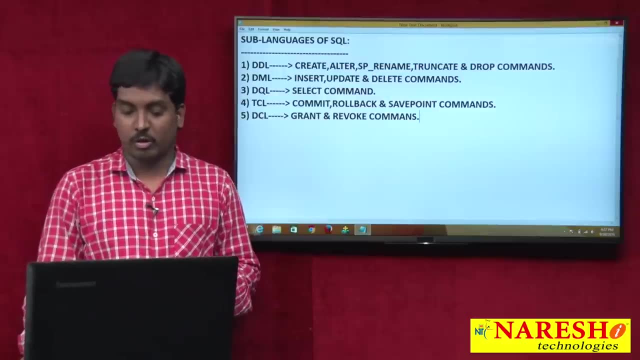 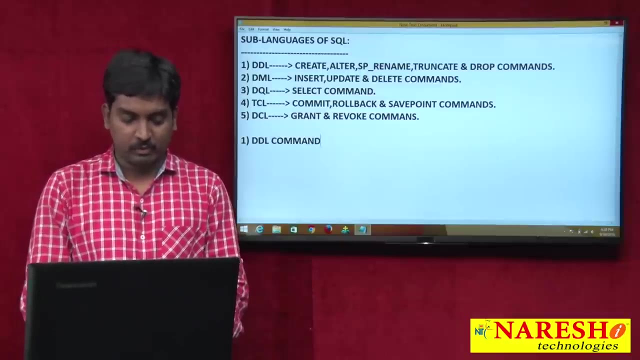 and how to use these commands and how to write my syntaxes. that all we can check out. okay, In this my first language. we will discuss here data definition language. okay, So now we will go to discuss my first one here: DDL language commands. 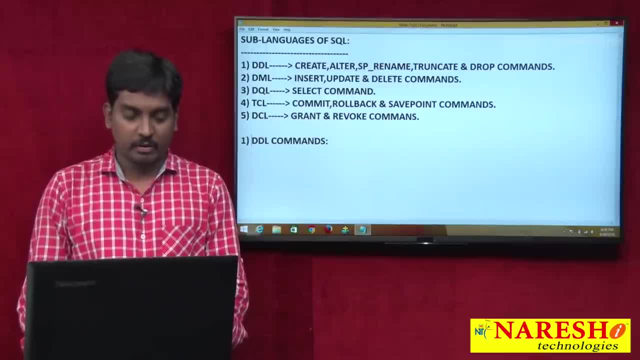 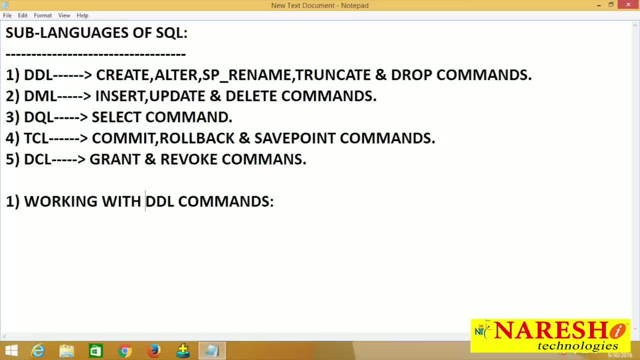 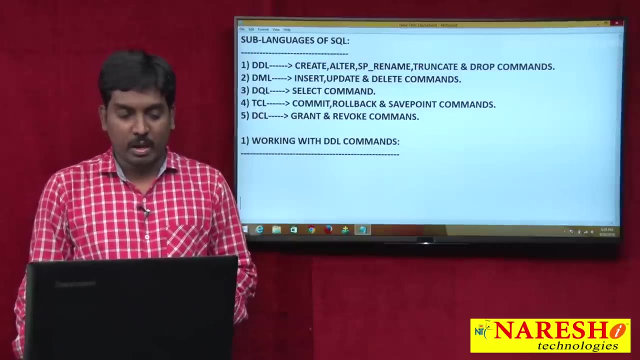 So DDL language commands and simple I can say: working with my DDL language commands, Working with DDL language commands, okay. So now in this- okay, I already said you this language was having total five commands. are there okay? 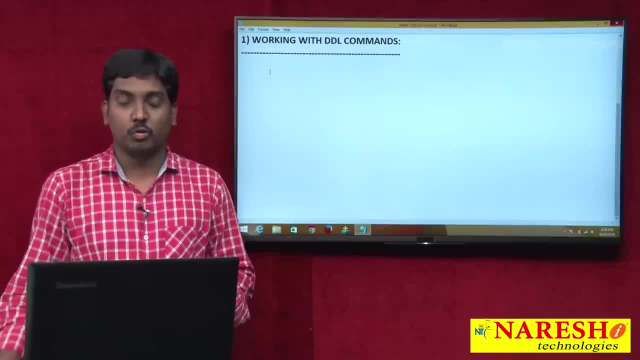 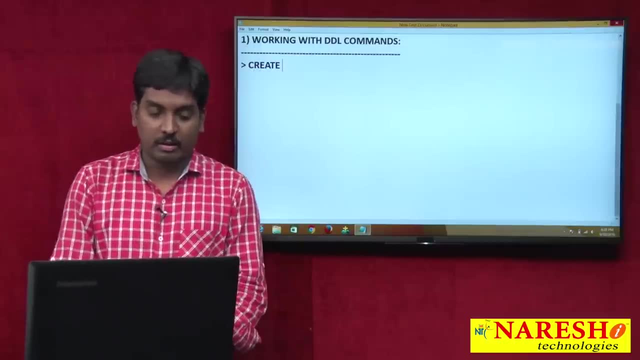 But here these language commands. basically, we are going to using- okay, for the three reasons I am going to using here. My first reason: what it is here? Creating or create new objects- okay, creating new objects? okay, objects are nothing but. 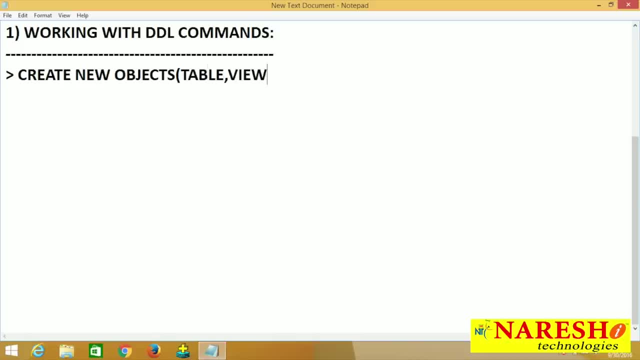 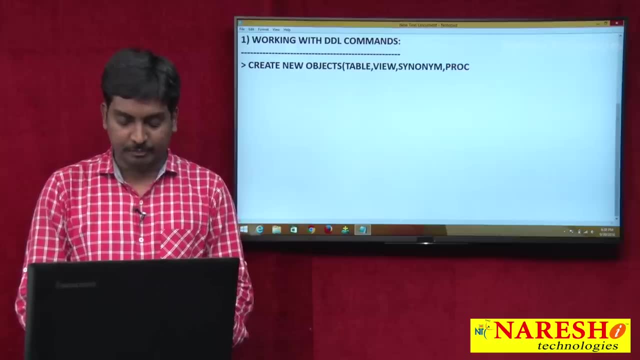 what it is here. For example, if I want to create a table, okay, otherwise, I want to create a view, otherwise. I want to create here synonyms, okay, Otherwise I can take your procedure okay, like functions, okay, and like triggers, okay. 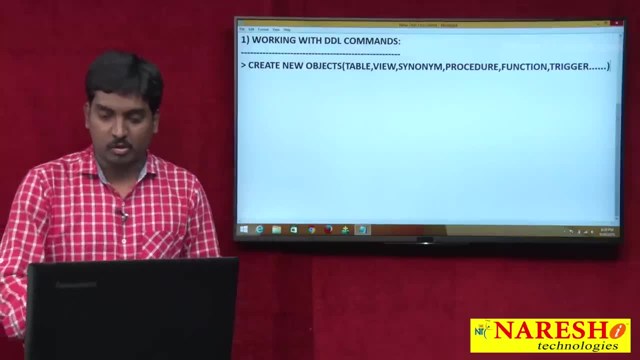 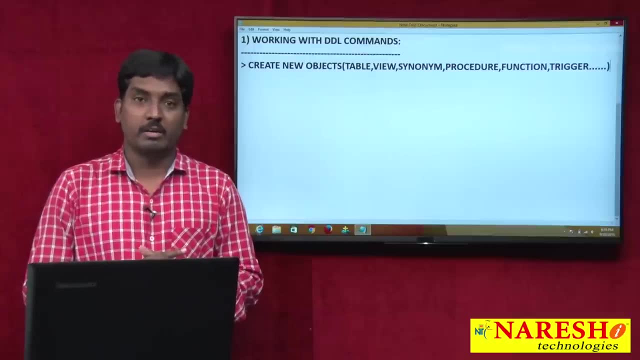 So, etc. These kind of objects I can go to create now. So. So whenever I want to create my table view, synonyms, procedure function and triggers, then you can go to use your DDL commands now, okay. So this is one thing why we want to use. 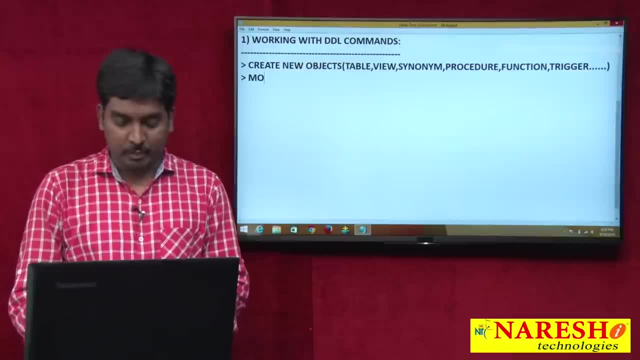 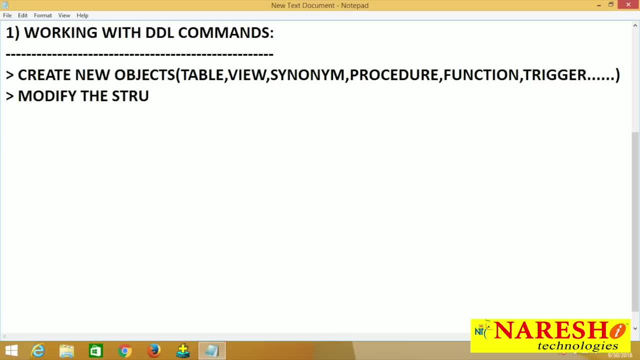 And the later next one. the second purpose is what now? The modification purpose? okay, that is called a modify. okay, The modify, what I want to modify here, structure, So I will be modify here. structure, so structure of the object or table. 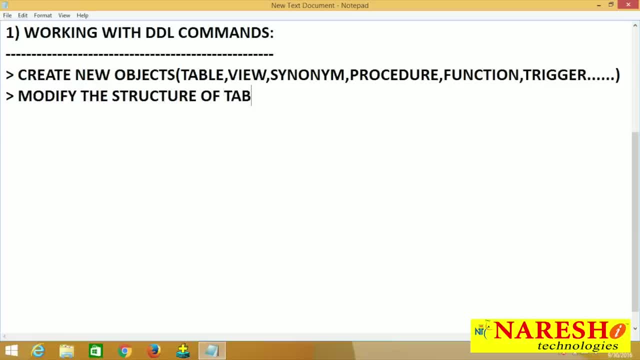 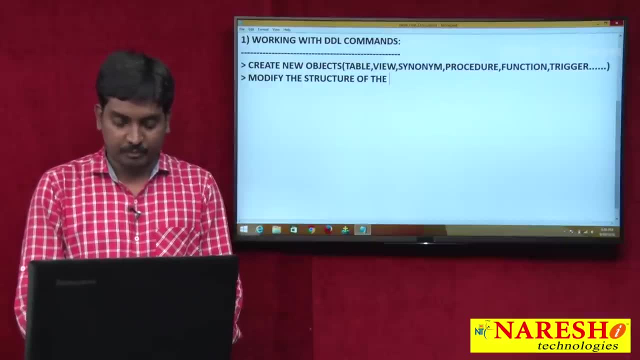 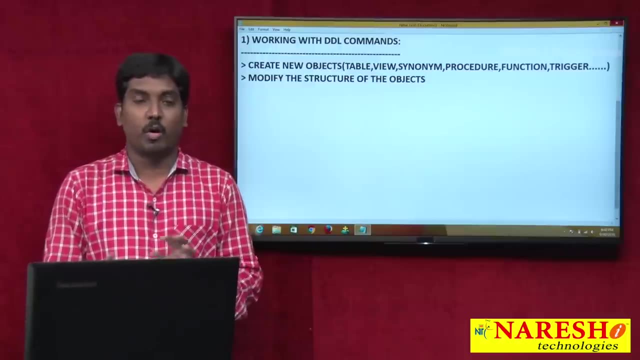 So, for example, I can say now The structure of a table: Okay, otherwise, any object if any object, otherwise I can simply say that structure of the objects: okay, the objects I already given above. So the structure of the objects, whenever you want to change is nothing but modify, okay. 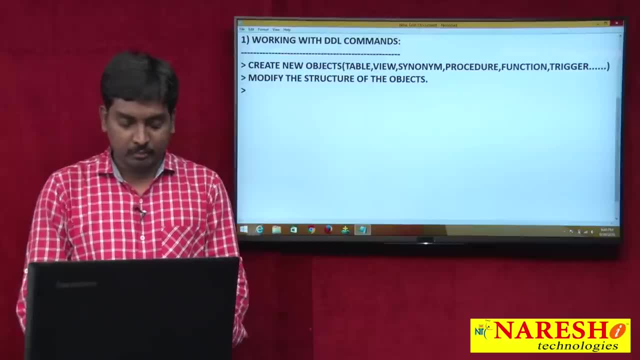 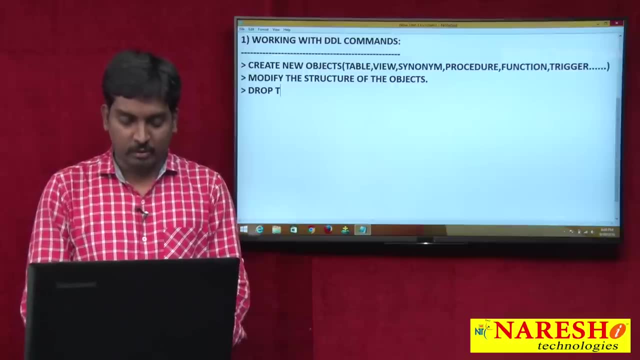 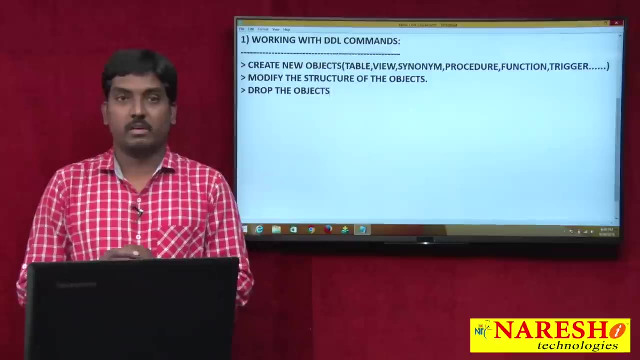 Then I can use it. And the next one, what it is here, then I can use for drop. So I can say: drop the objects, okay, dropping or dropping the objects here, So I can use my drop objects. So whenever I want to drop the objects from database, I can say: simply: from database even. 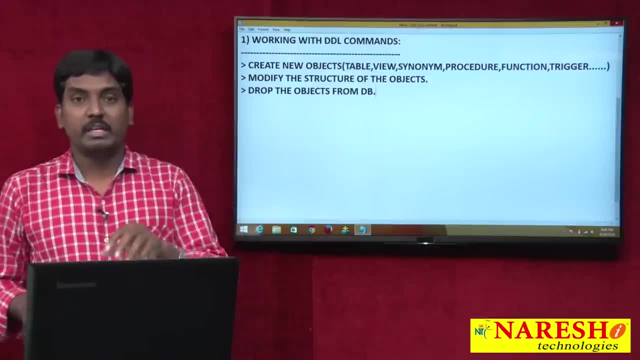 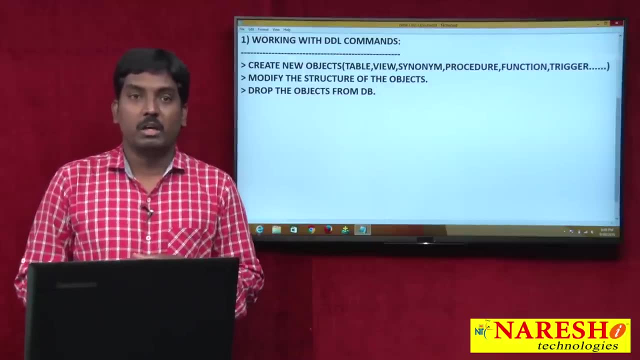 though I can use my DDL commands- okay, So that means DDL commands- the basically we are going to using for the three reasons. One is creating purpose, creating objects and modify structure of the object and later dropping the object from database. 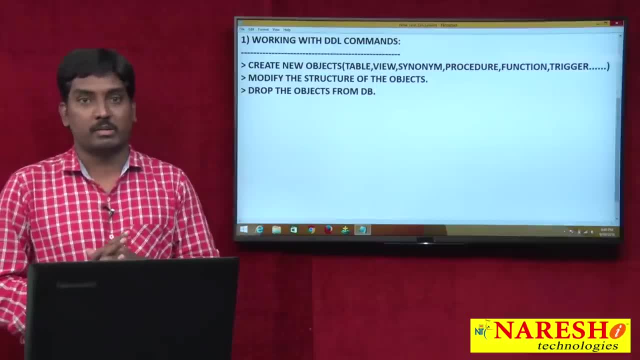 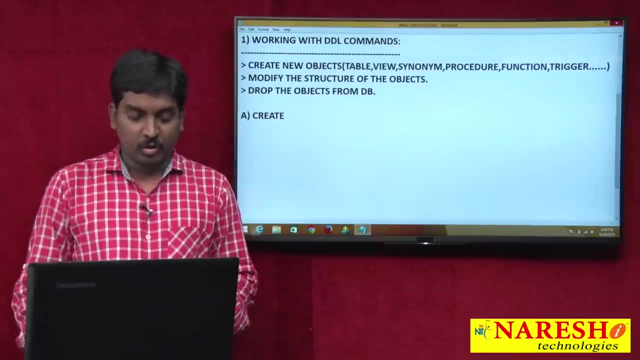 So these are the main reason why we are going to use DDL commands. okay. So in this, the first command we will discuss here, my first command is what now? Create command okay. So I think all of you know your create command okay. for what purpose I want to use that. 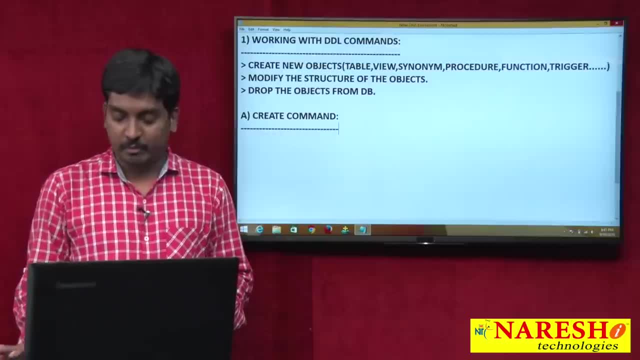 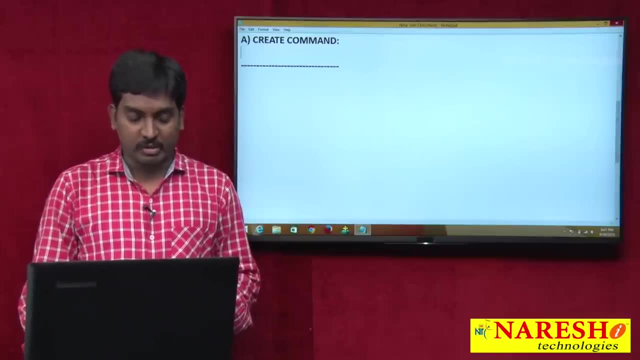 everyone know this. okay, So create command simply. I just say okay, create command. simply. I just say this command is used. okay, this command is used to create my objects and also database. So whenever you want to create your new database, even though I can use my create command, okay, 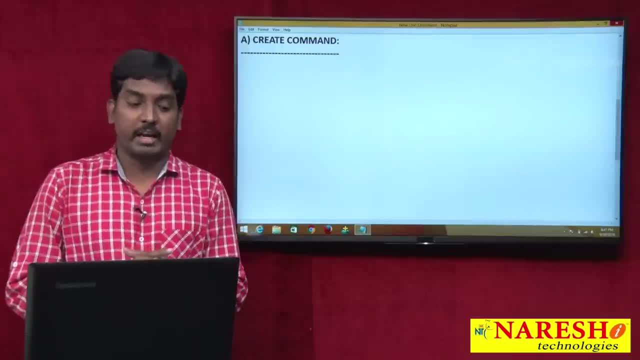 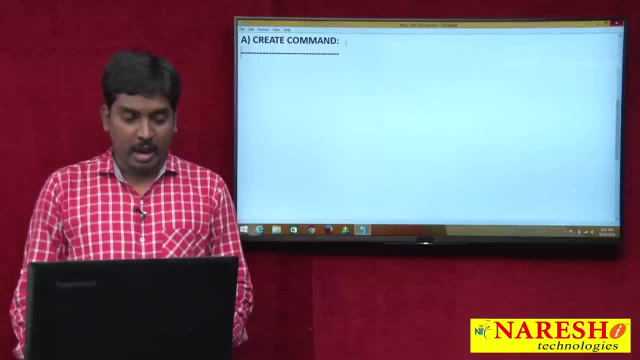 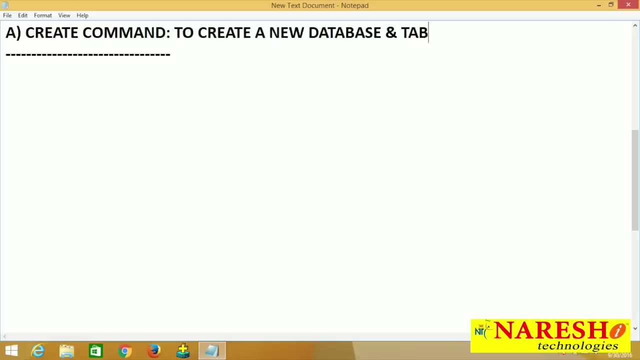 And also objects is nothing but table. If I want to create again, I want to use my create command. okay, So this command using for to create a new database, okay, I can use to create. okay, to create a new database. okay, create a new database. and also like objects are nothing. 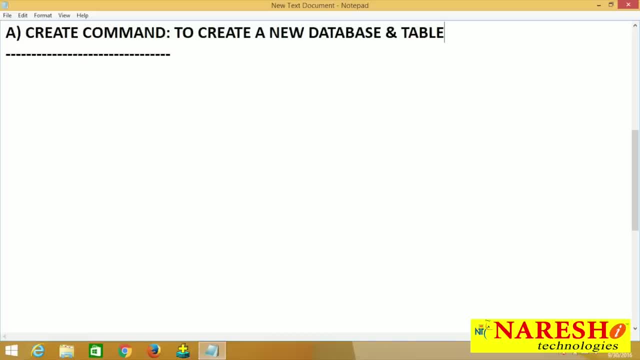 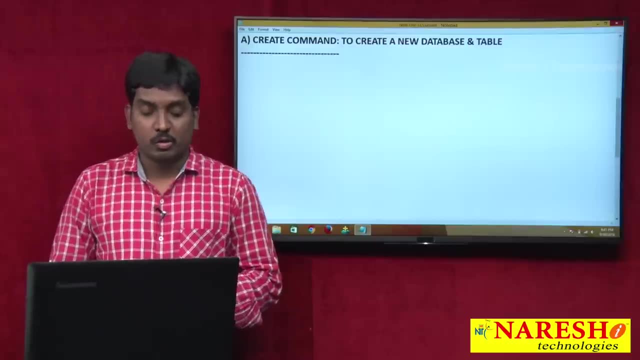 but what now? Table I create to create a new database and table. Okay, I create a new database and table again. I can use this. okay, create command now. okay, So now, first of all, what I want to do before I want to create my table, first of all in: 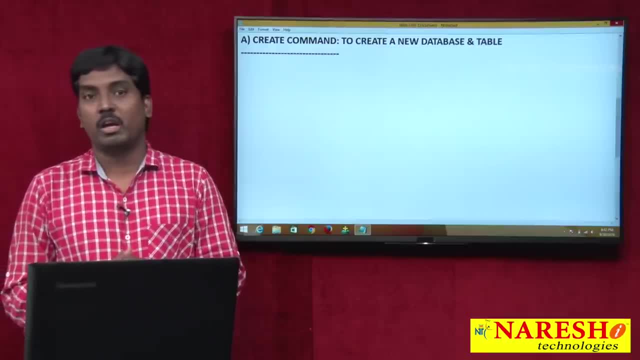 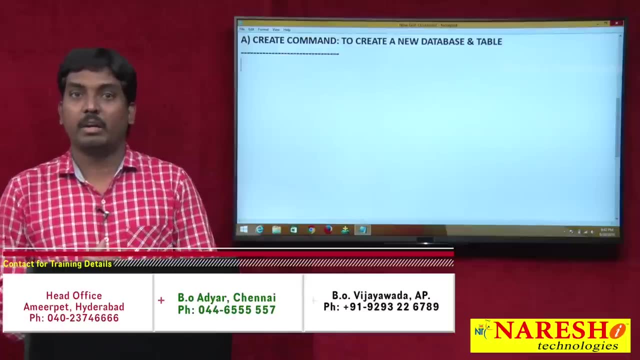 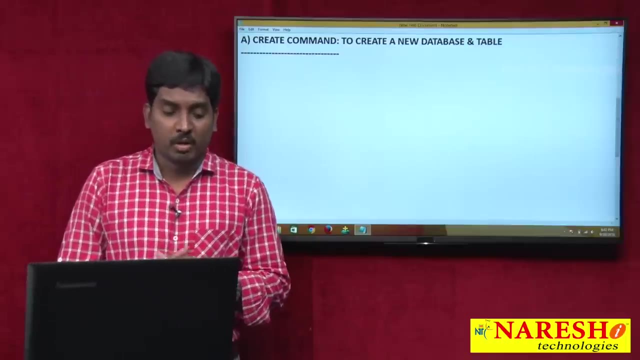 my SQL server. first I want to create one database. okay, So after creating database, later in that database, later I want to create my table and after creating table, then later you can go to perform and go to insert your data or update or delete. So data manipulations you can do it. 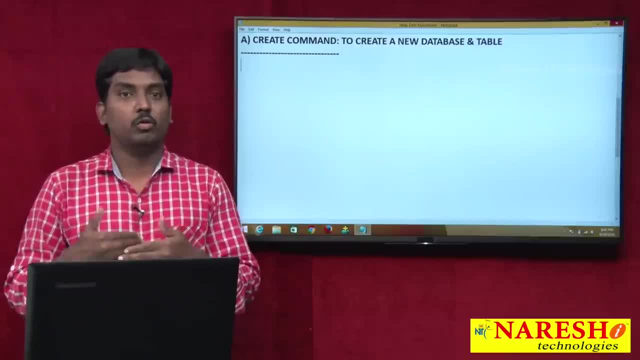 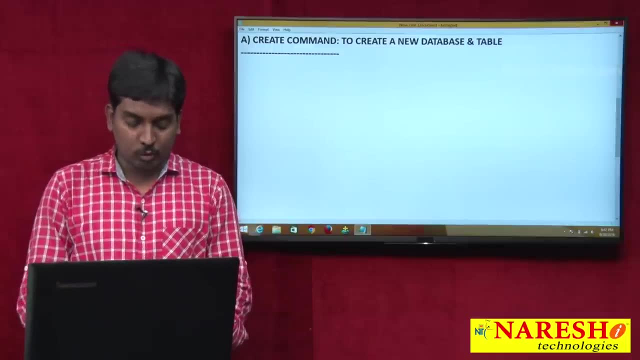 So, first of all, what I am doing here? Okay, First, in my SQL server, I will go to create one new database. okay, and later I will create one new table in the database. okay. So, for those purpose, for those operations purpose- I should be know the syntax- I am going. 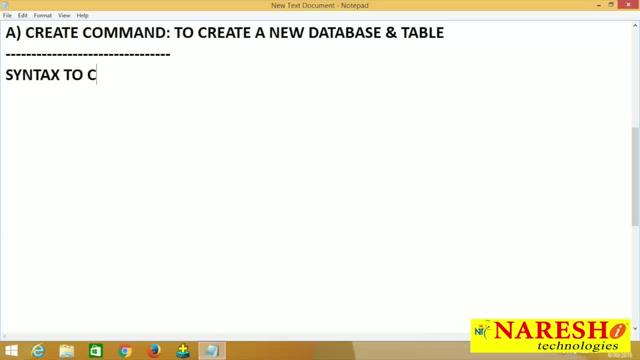 to showing here the syntax to create the syntax to create a new database first of all. So I am going to take here a new database first I am creating for this purpose. I am going to give some syntax to you. just you just remember, here The syntax is very simple. 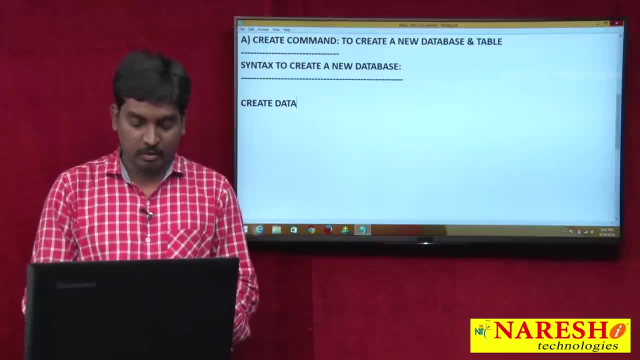 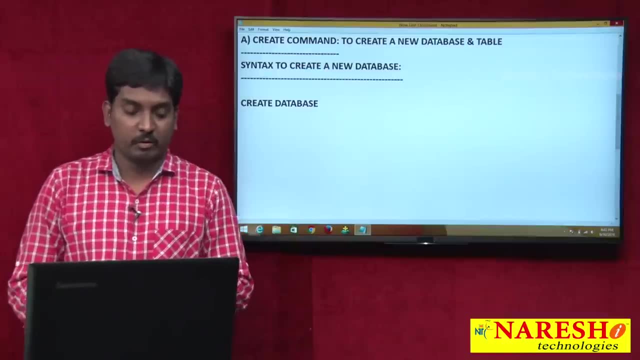 Okay, It is very easy. So create what I want to create now: database. So database is a predefined keyword. okay, So create is a command and database is a predefined keyword I am using and to create database. I want to send here database name. 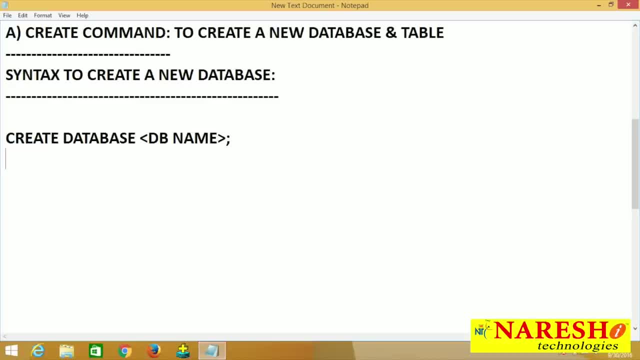 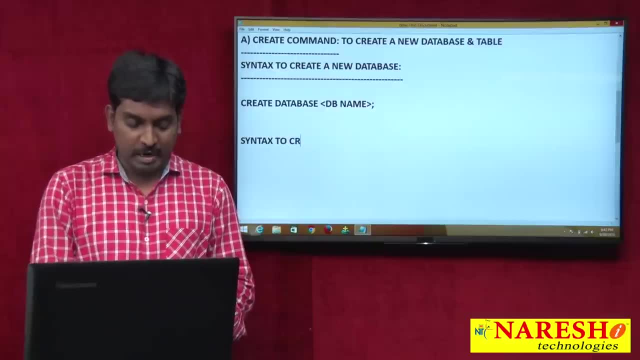 So this is my syntax here to creation of new database. okay, After creation of new database, what I am doing here later: how to create my table. So now I am going to writing here syntax to create, okay, a new table, A new table. 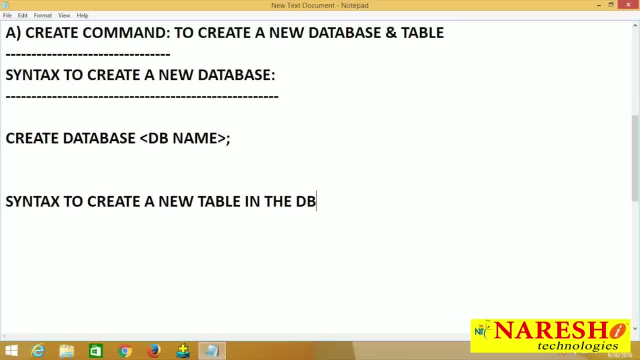 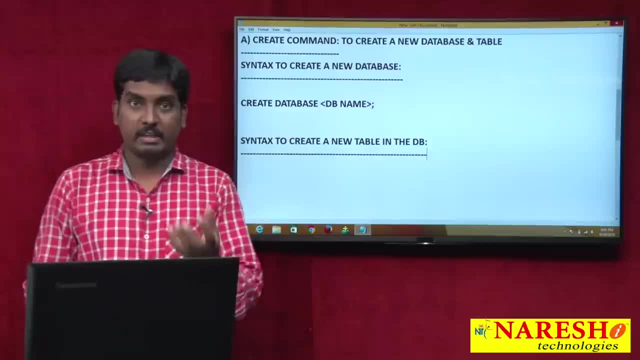 A new table in the database. okay, This is my second. okay, So how to create a new table in the database. So, whatever the database I was created in that, how to create my new table for creation of new table is simply called it new structure. 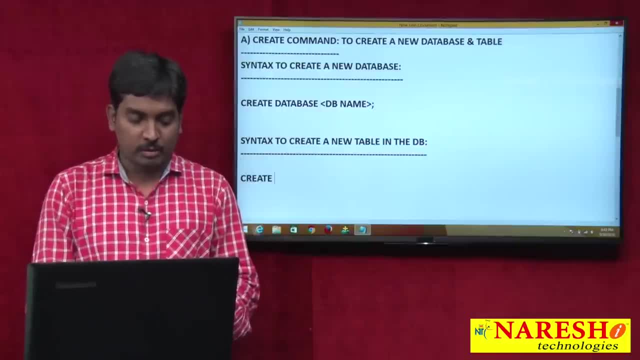 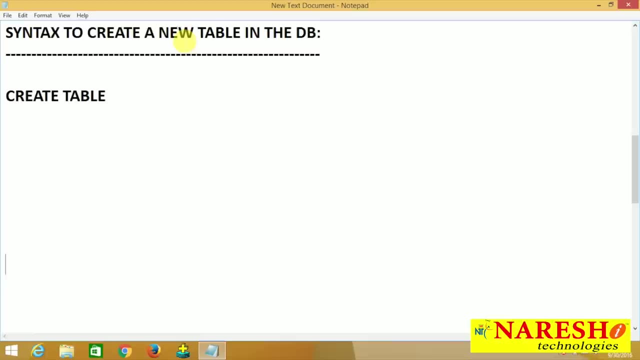 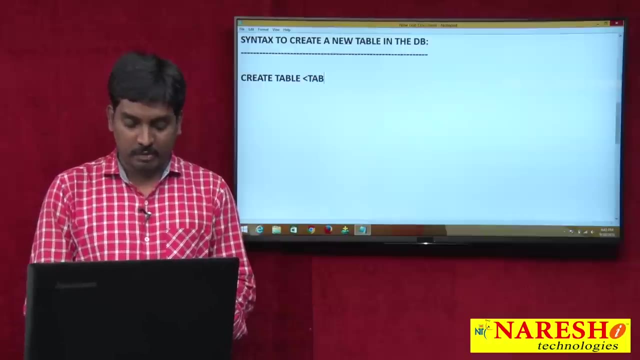 The table structure. if you want to create, then this syntax should be follow. what is my syntax here? create, okay, I will take your table okay. So create and table Okay Now. later I want to send here. I am passing your table name, so otherwise I will take your. 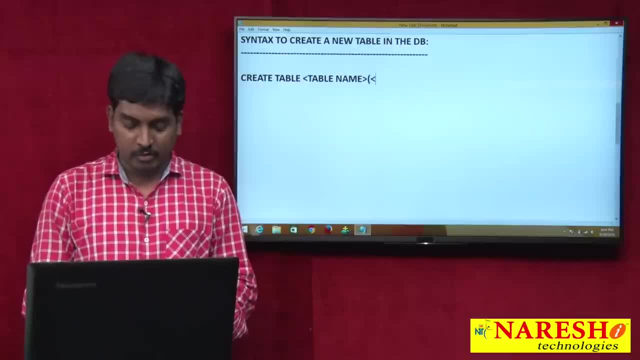 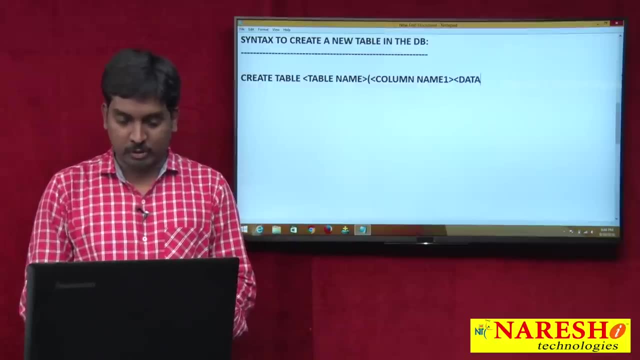 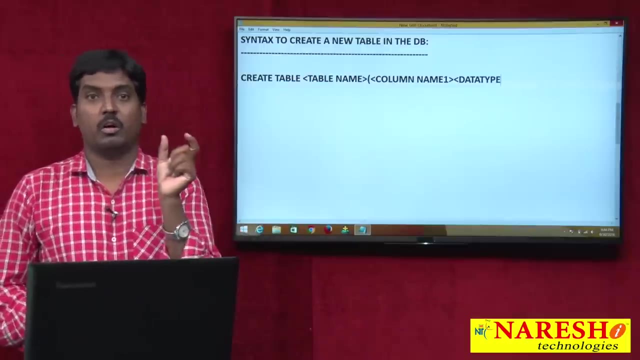 table name. okay, of then. later I want to send my column name, So you can send my column name one after column name, For every column name, after you just send your data type because you know that. okay, So this or the column is regarding to, or belongs to, which kind of data type that I was mention? 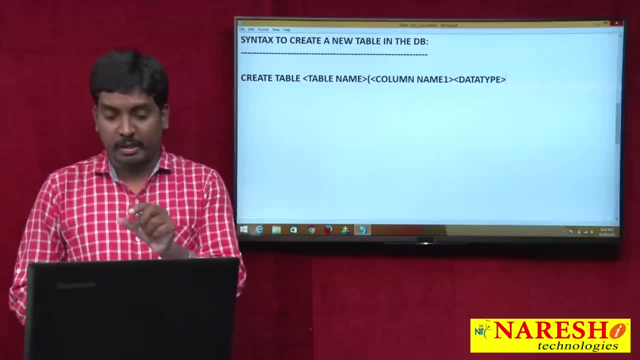 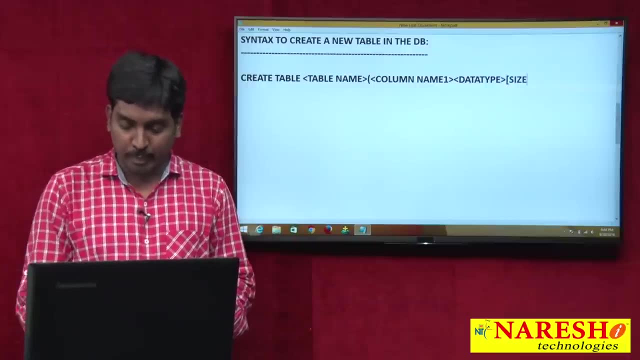 here am taking your data type, data type. So data type I was taken here after column name should be applied data type. If the data type is a character data types, then you should be mentioned size. ok, So the size should be mentioned when your data type is a character. 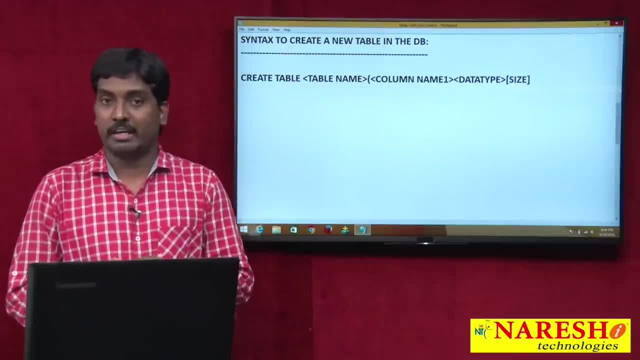 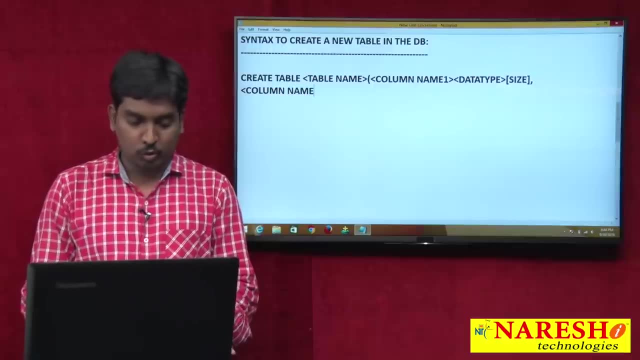 ok, otherwise, do not mention the size of the data type. ok, So like this what I am doing here: the column 1, comma, in the same pattern. if I want to go for my column name 2, ok, the second column I am creating in the same to same. I just send my data type and if it is, 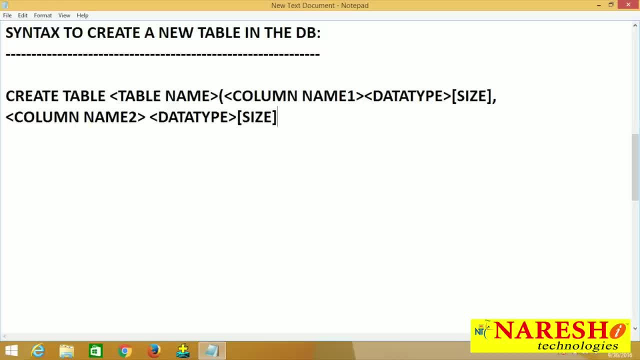 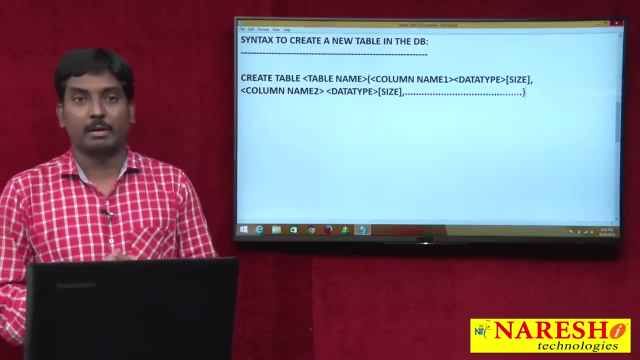 a character data type. what I want to need here: size is required, ok, So comma and so on. So, like this what you do, like this, you can create number of columns in a table, ok, So just, I was created. thus, two syntaxes I am showing in this, ok, One is how to create: 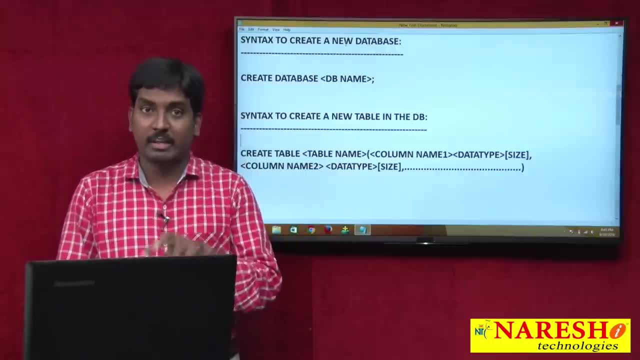 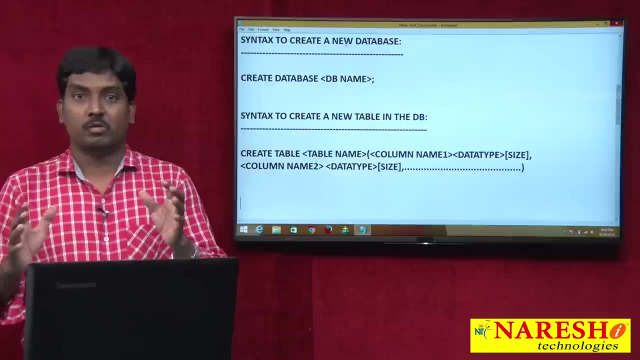 a new database and later how to create a new table within the database. ok, So by using this two syntaxes, now I will go to create my database, So database and table in SQL server. ok, So how I can create? ok, by using this syntaxes: 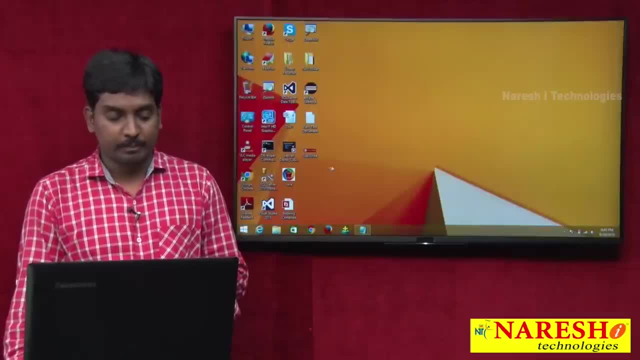 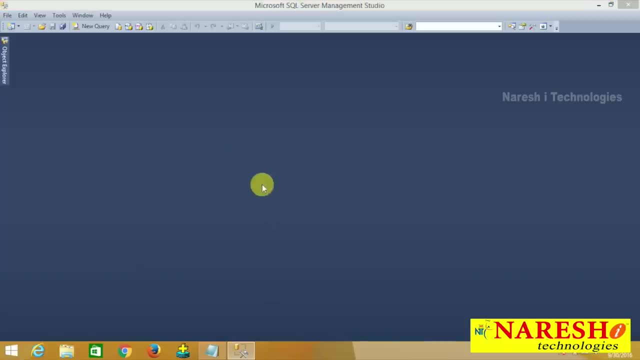 you can see now. So first of all you will be go as usual. ok, go to open your SQL server management studio. ok, that you know how to open SQL server management studio and later I just connect. but I am going to connected. ok, I am going to connect here. ok, connecting. 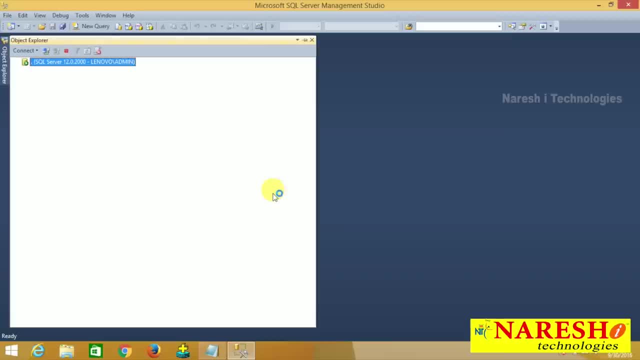 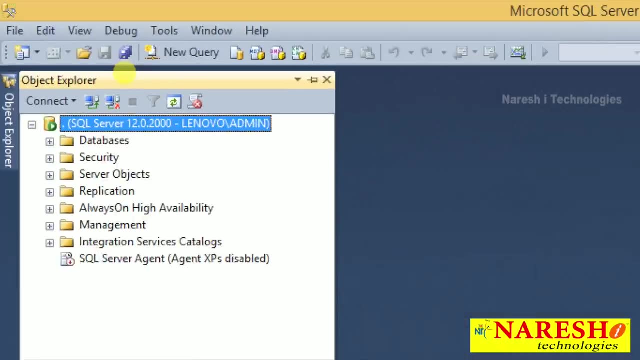 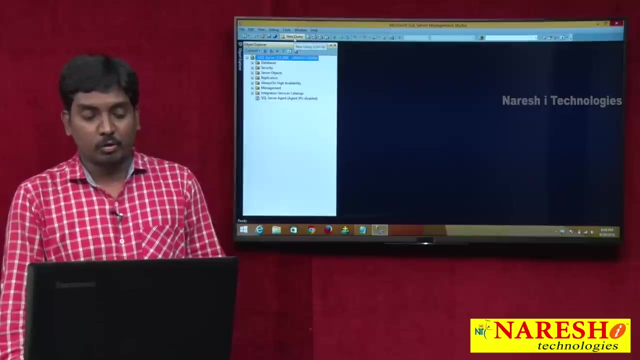 to my SQL server with the windows authentication is nothing but administrator. So I am admin. ok, So I already said to you, admin means I can do anything or any kind of operations I can directly perform in my server environment. ok, and now I am going to take here. So to: 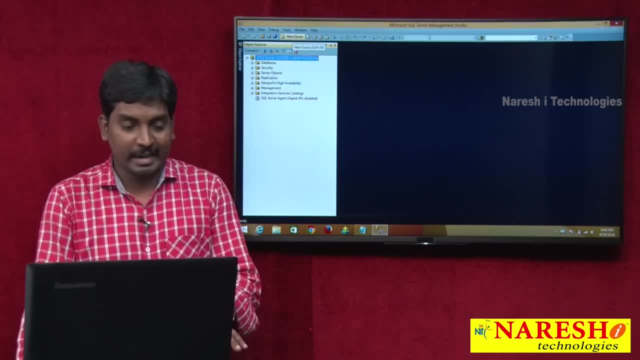 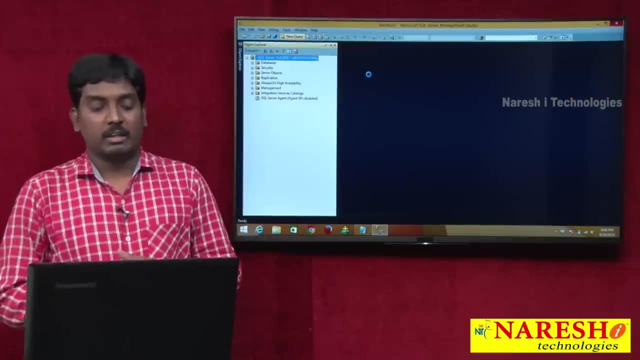 write my query, I need a query editor. that query editor we will be take with the help of what now? new query option, So I just come out to click on new query option, then that new query window will be open now and later on. later on what I want to do, I will be created. 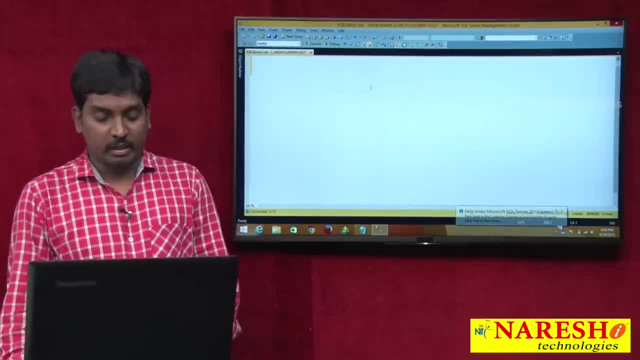 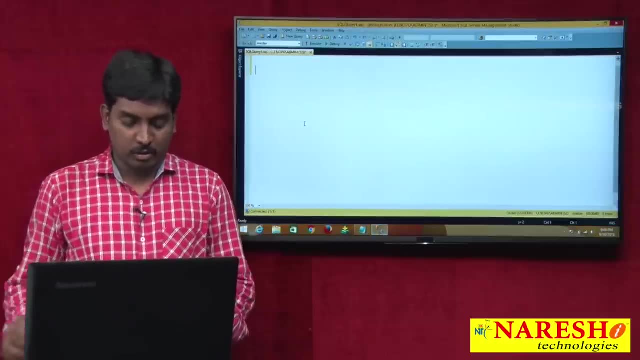 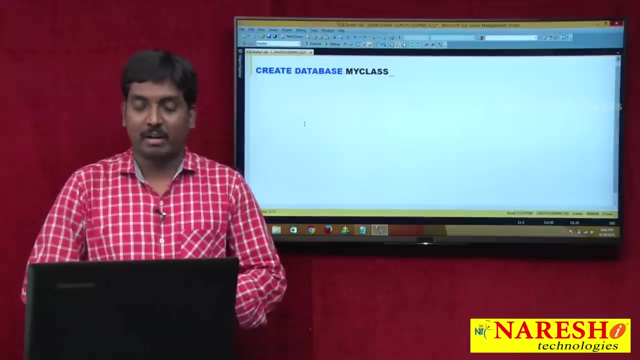 one new database first. So syntax. already I was given now the syntax: create database, database name. So now later I just come out here to created one database now. So create database, my database. now So I can say my class, ok, So my class is my database name. So after writing your syntax, 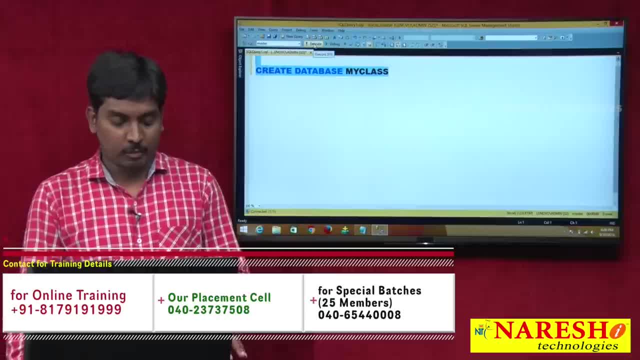 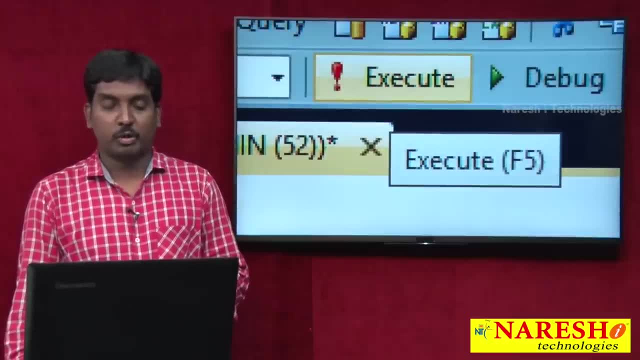 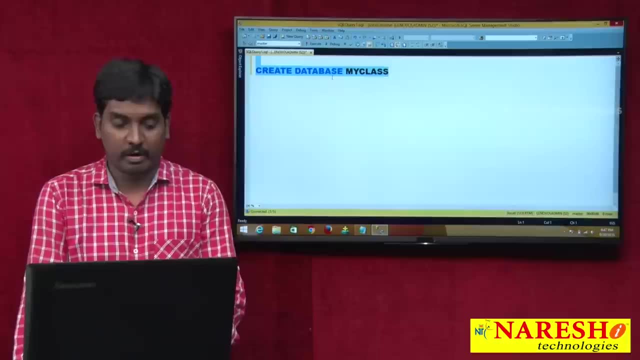 you just select this entire query and later you just come out and click on what now execute option. And I already said to you, whenever you want to go for to execute, either execute option you can use, otherwise F5 keyword you should be use it. So now I just selected this entire query and to click on F5 keyword from my keyboard. 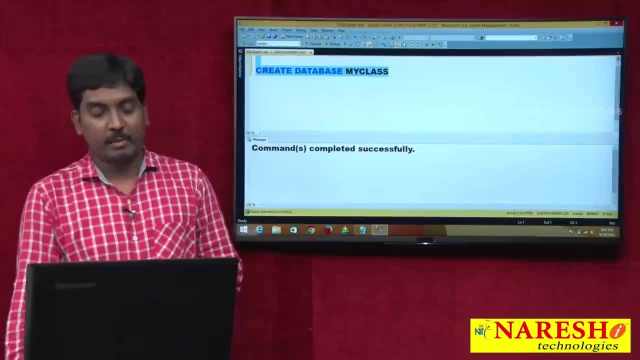 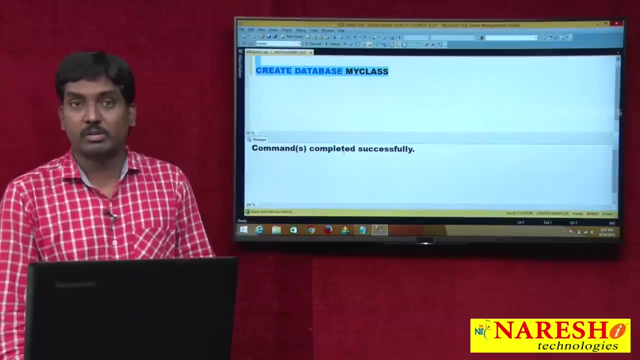 ok, just I enter. After enter what it is happen, you can see command was completed, successful. ok, So later this command, this statement, whatever the statement you got, it means this is a positive statement. that means your query successfully executed in my server. ok, After. 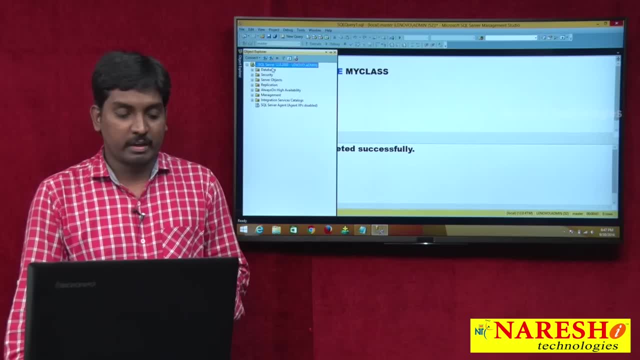 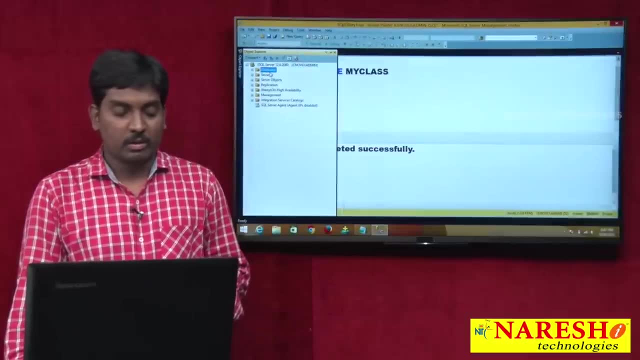 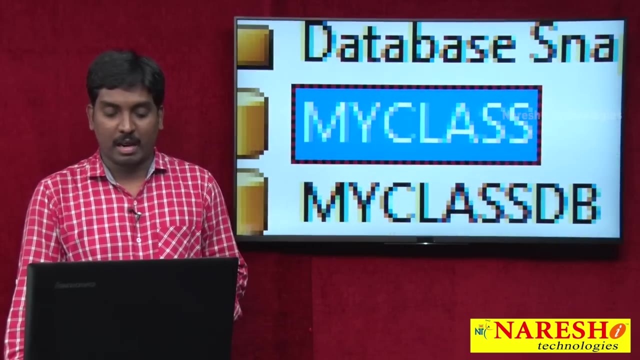 executed what I want to do. This database was created. This database was created. So let me come out here and see this heading. so this page, we need to 아 ένα pieces from beside window. these document. I want to see all this one. ok, are these two case samples? 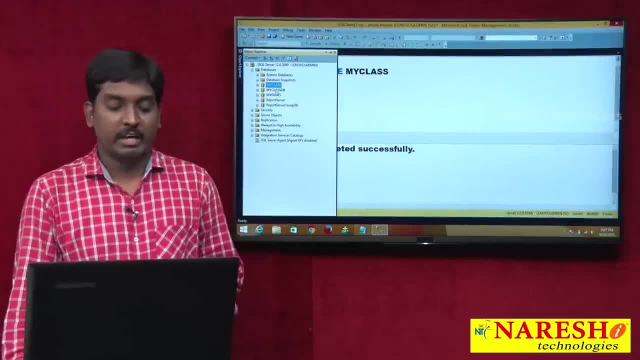 ok, I want to see this folder, So let me just turn it on. ok, that means I have created one in thatido. Now let me see how open this one now. So what is called? say in that you have not your user named, your. 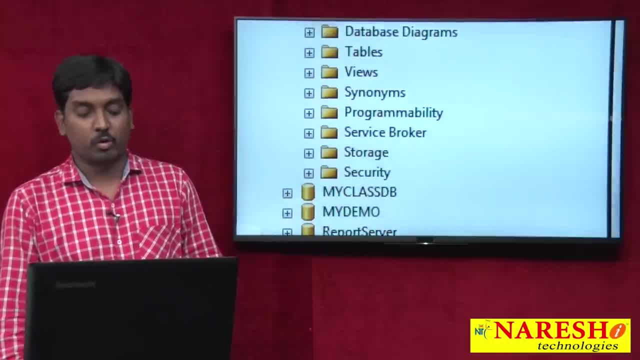 user profile located in this page. So in this question you might have to access the details on you, So you cannot there then when you want to have the name and if there any detail, that and security. So in this we are going to discussing with what now tables. So, but here, 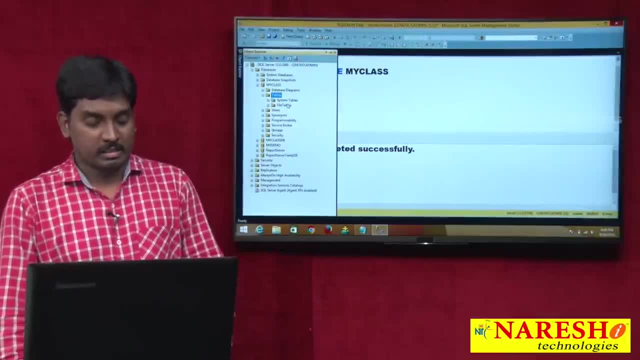 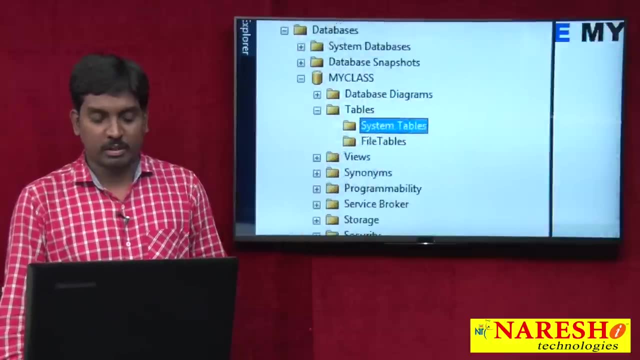 you just come out to open the tables folder. Here system tables and file tables are there, but these are not necessary here. I just open this folders also, but there is no system. there is no file tables, The system file tables. how to create that we will see in the later. 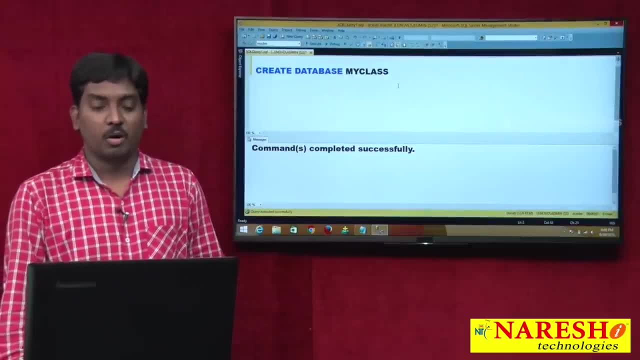 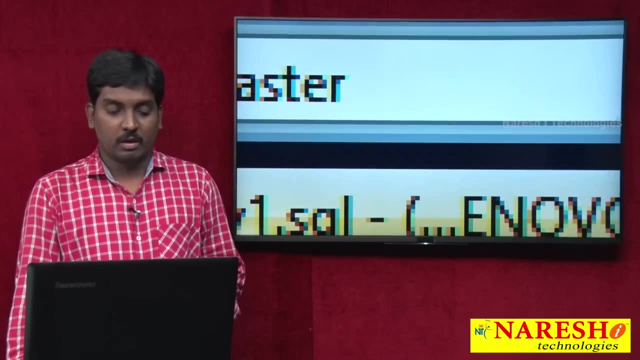 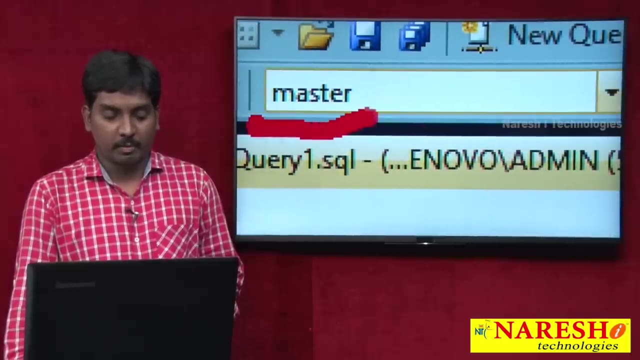 session. But here I just go to created my table now. But before I want to create a table, first thing should be remember. So first of all, when you see this drop down list was there here. In this drop down list, control automatically by default, the database name was there. So what is the database name? was there here, master? 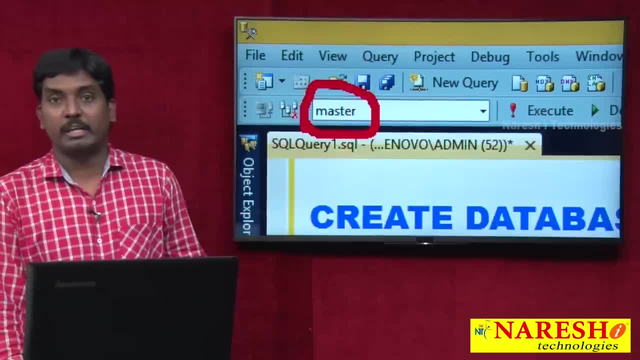 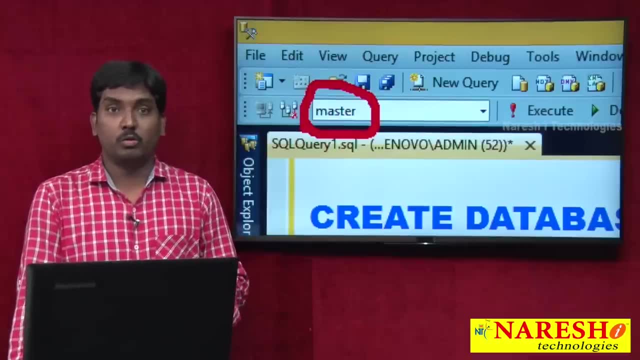 So that means if, later on, if you created any new table later on, if you created any new table, the new table was created under master database. So that is why what you want to do, So this table should be create under my own database. So what I created now, what is my? 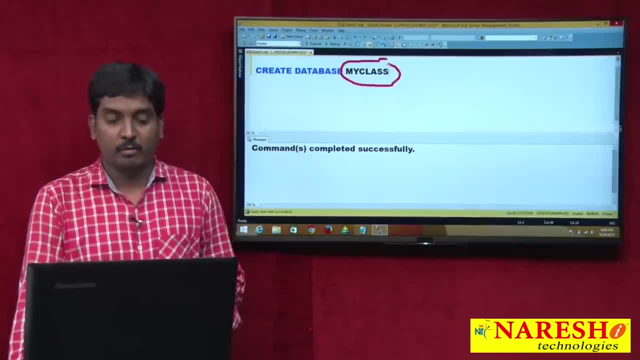 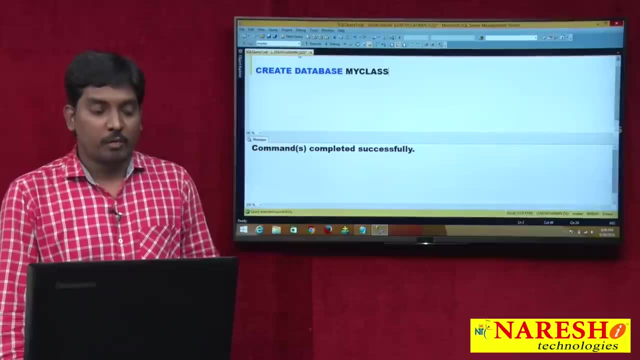 own database here, my class. This is my own database. I was created, So into that database I want to store my tables, So to store, like this, what I want to do here. first of all, the two ways you can go it: One is I am going to using through query, How to use query means. 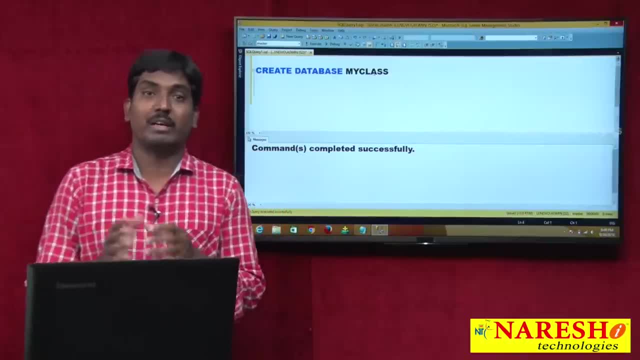 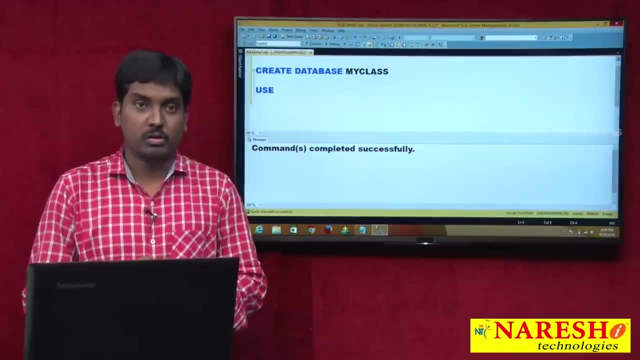 first of all, in which database do you want to store your tables? First, the database should be selected. For the selection purpose I am going to use query, So first of all I am going to using now here, use and use keyword, use So database name. what is my database? 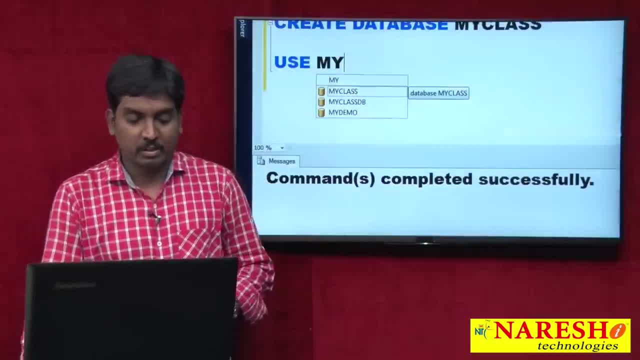 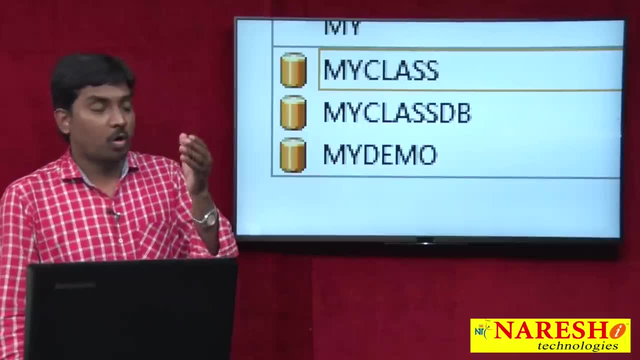 name, So my class. can you see this once you enter like this, automatically in your intellisense box your database, that means how many databases are available in my SQL server, So that all databases are showing now. but in this my class database should be selected, because 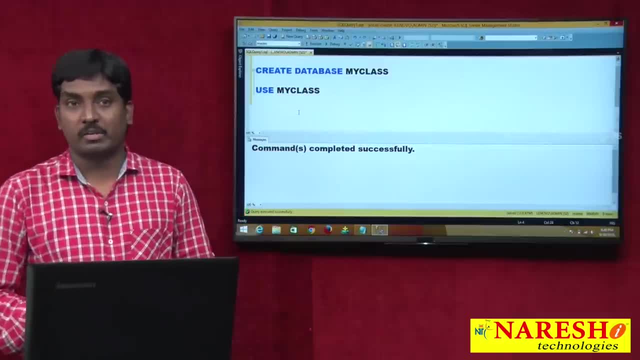 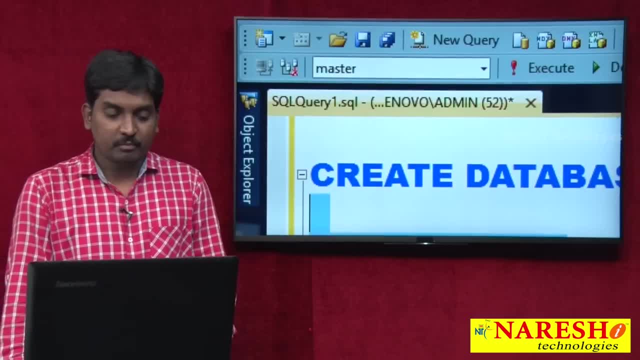 keyword. So I am going to execute now this keywordSo I am going to execute now this keyword. So I am going to execute now this keywordSo I am going to execute now this keyword. So I am going to execute now this keyword. So I ع 대. 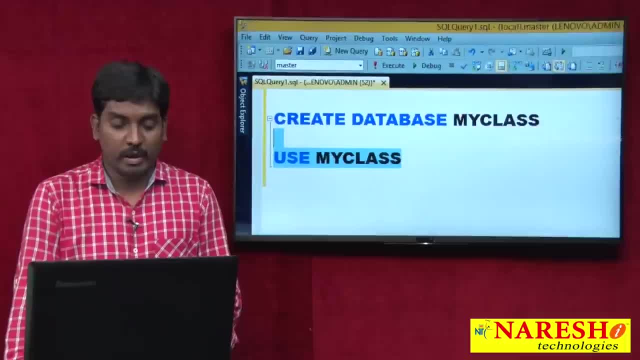 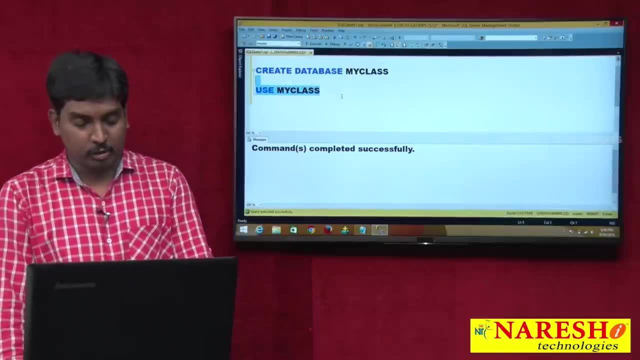 So by default, master was there, but when I want to execute, use my Class statement, then which database was selected there user is come out and check. Now I go to executive. now, Once it was executed, command was completed successfully and did you identify here? So 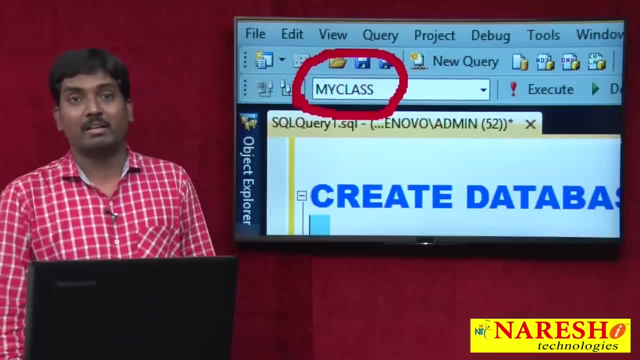 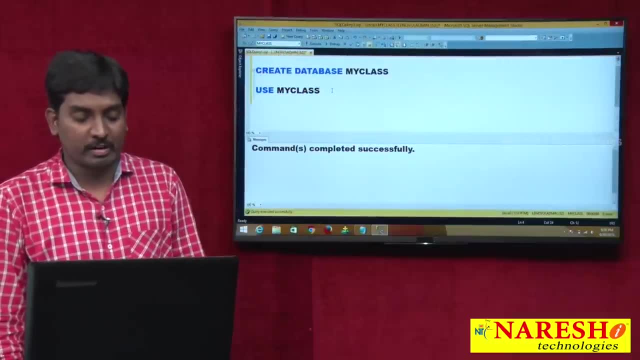 in place of master what it will, it was came my Class. So that means now I selected which database I selected. class database I selected through my query. this is query through I selected. Otherwise, if you want to directly go to select your required database from this drop down, 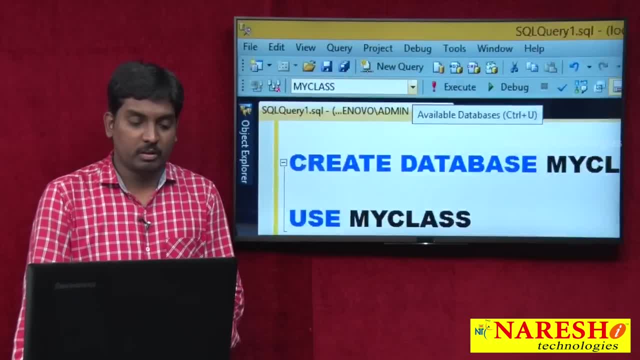 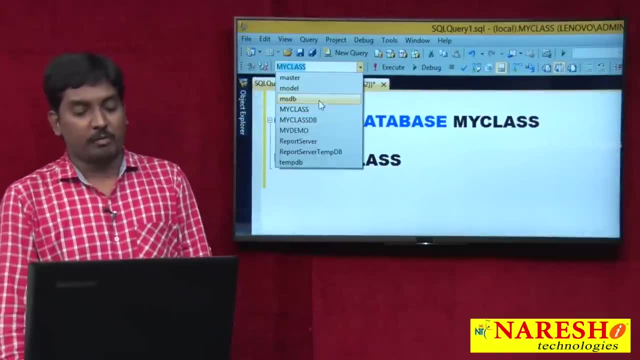 list. then you just come out here and I just drag and drop. just I am going to drop now Once I want to drop here. then it was dropping now after dropping in your server. how many databases are there? that all databases here showing now? 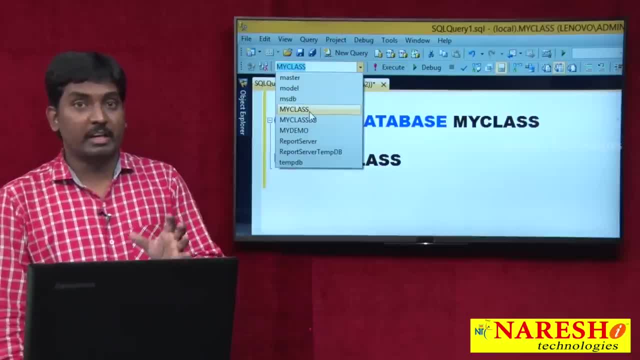 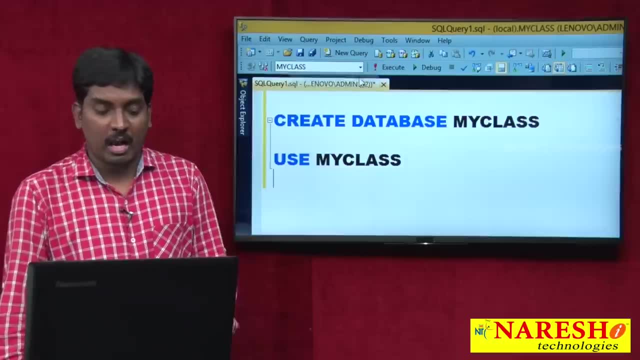 After that here: which database, in which database do you want to create your table? the database you should be select. So even though you can select like this also. So my class was selected here, otherwise you can change. see next. I will select my demo. 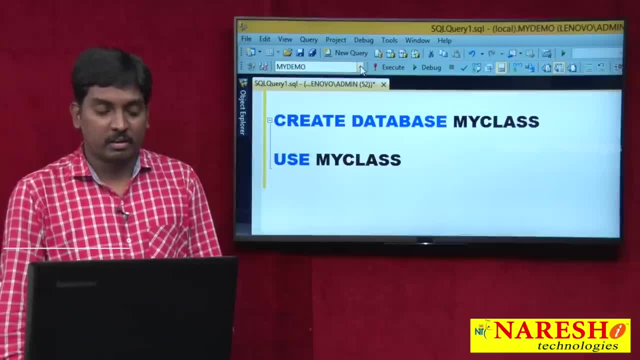 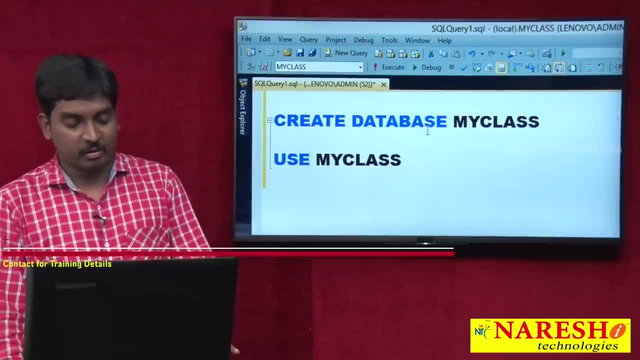 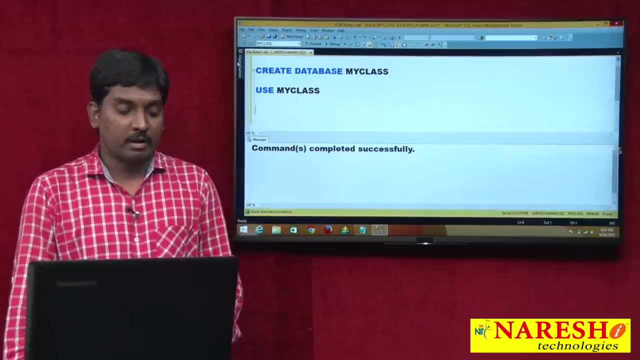 So now it was change my demo or not. yes, So in the way directly you just go to. so to select your manual database, which you wanted, After selected my database here, then later what I am doing here into this database, my class. So I am going to create a table, but in my class database I already open my table folder. 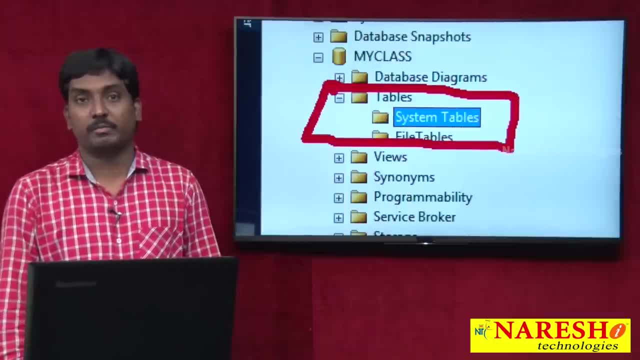 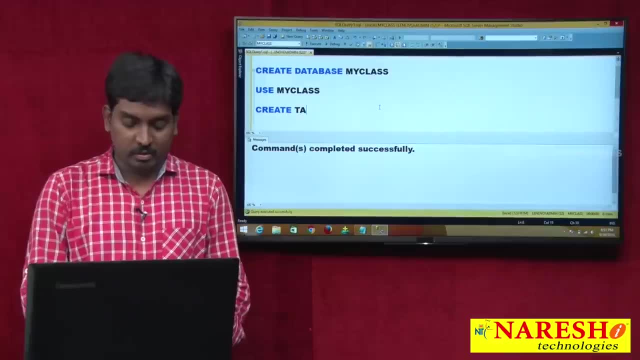 So, as of now, there is no tables in this database now. So now what I am doing here? I am going to create one new table. So the syntax. so what is the syntax here? create table, table name, for example, simple. I can say: my table name is employee. 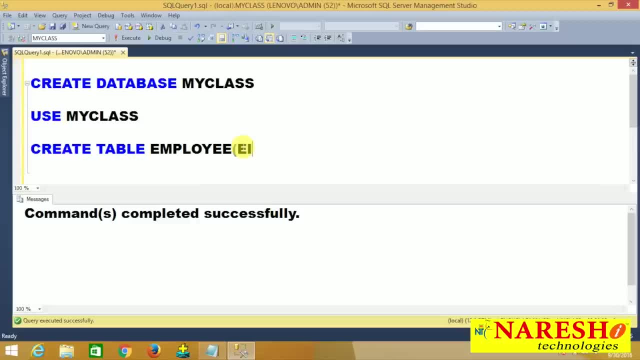 I was create. my table name is employee and I will send here employee id, So employee id, integer, data type And later I will take employee name. So otherwise simply I can say emp id, integer, So emp name. I am sending here the varchar of so otherwise, in place of varchar, first I will 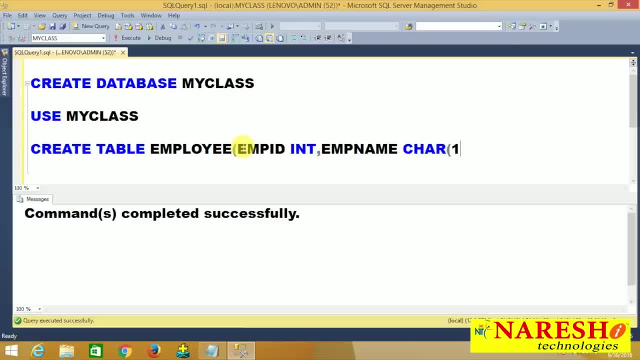 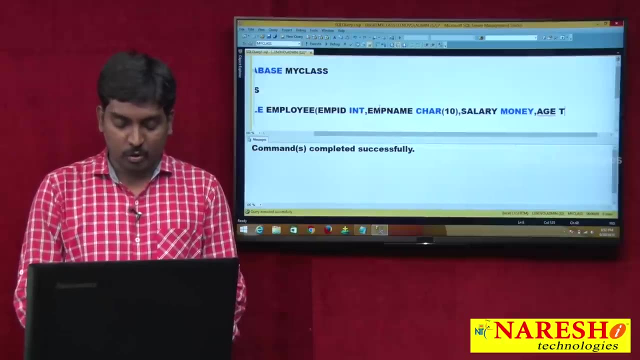 go to create my ename or emp name with the char data type I created and later I want to take here salary column with one more data type- was there that is called money. And later what next? for example, after salary I was taking age, So here age. you want to use integer, otherwise tini, int, whatever you wanted. 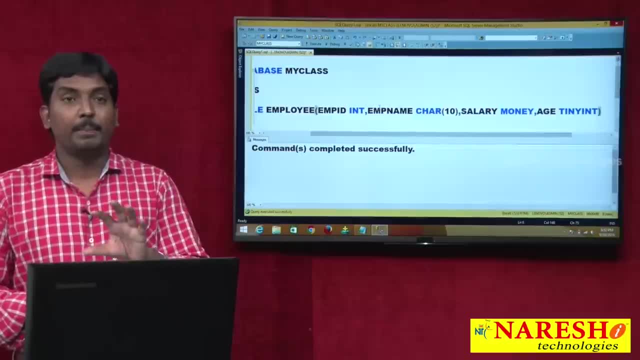 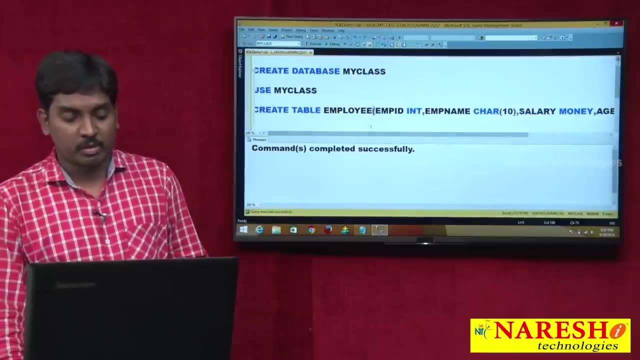 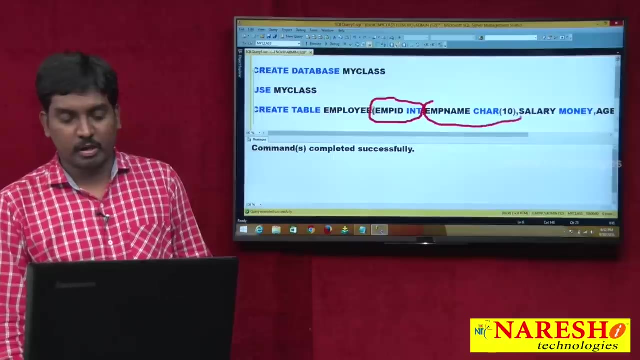 So like this what I am doing here. here I was created one simple table. the table name is employee with the four columns. So whatever the column names, here my column names are. one is eid, column name with integer data type and later ename with char data type and later salary with money data type and. 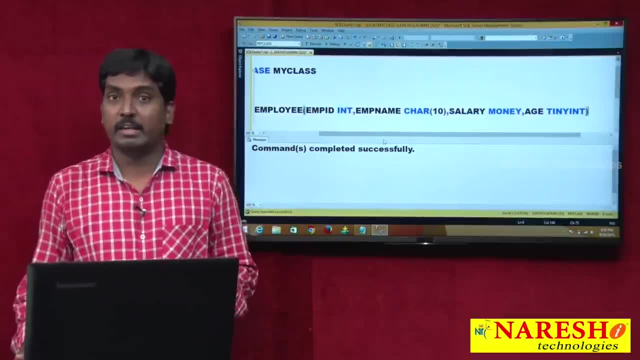 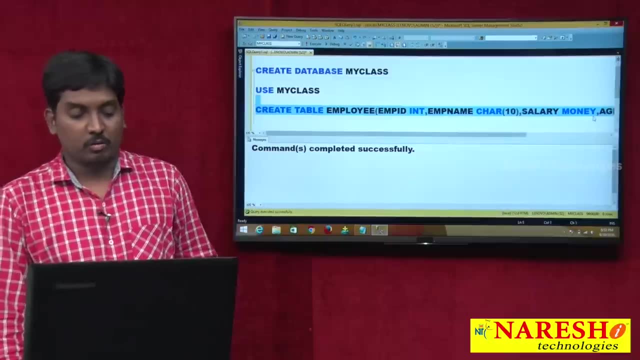 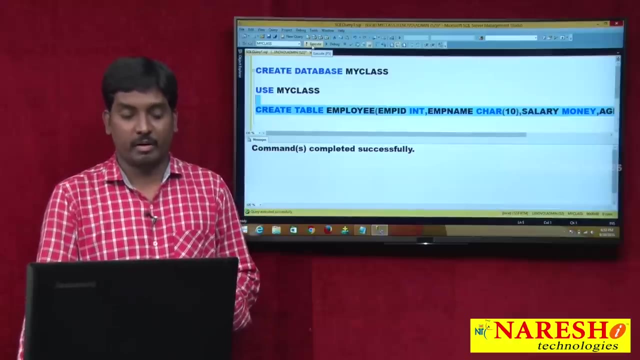 finally, age column name. This column is also having integer data type that is called tini int. So these are what it is here: the table creation and columns. Now the complete query I just selected here. after selected, you just come and click on execute button. otherwise press F5 key. 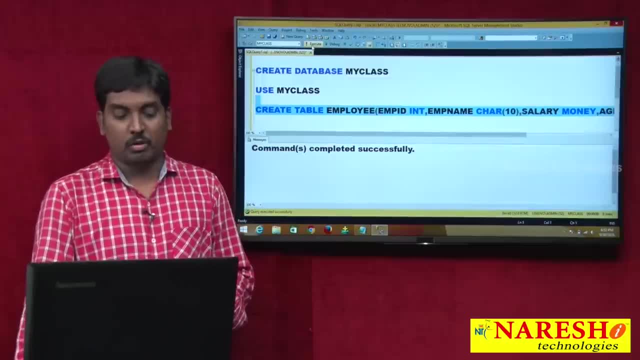 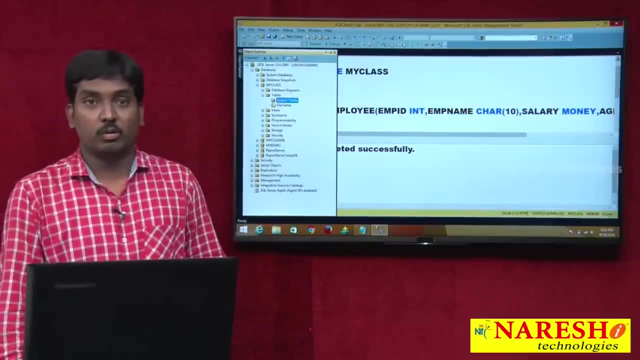 So once I go to execute now, once you can go to execute now, command was completed successful. After command was completed successful, then what it is happened, if the table was created or not, you want to check For the checking purpose, what you want to do. 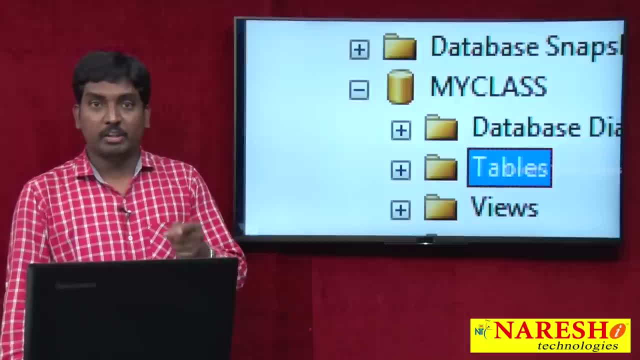 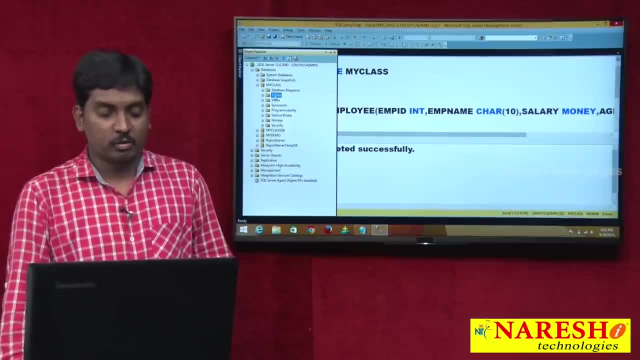 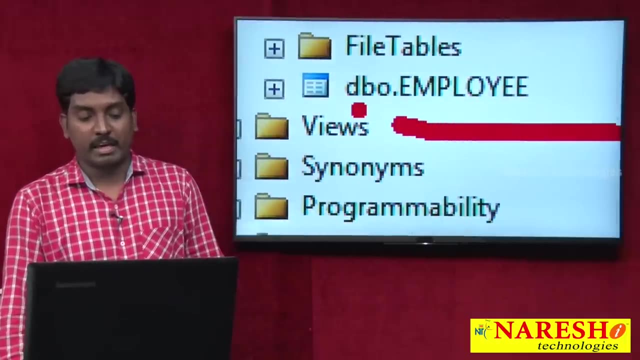 Go to your my class database, because in which database are you created your table? go to that and I just refresh my tables folder and later you just go to open. now, Once open here, the table was created with the name is what now employee? and your extension. 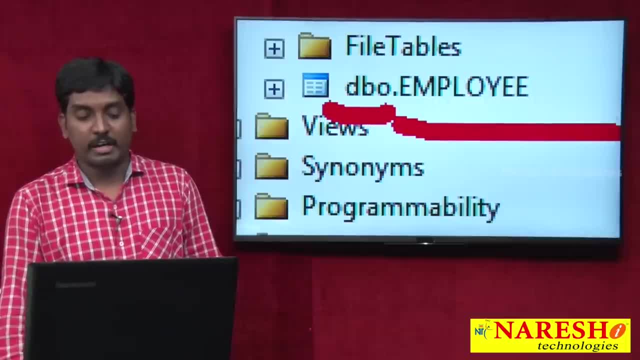 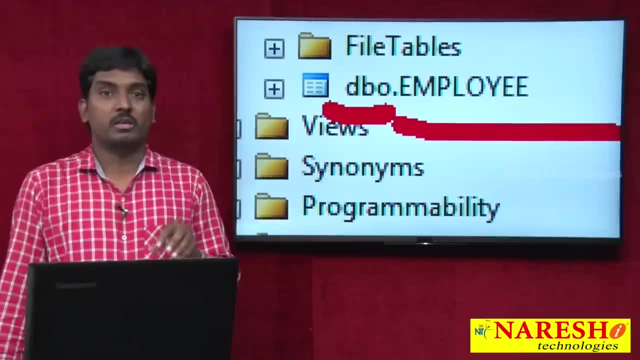 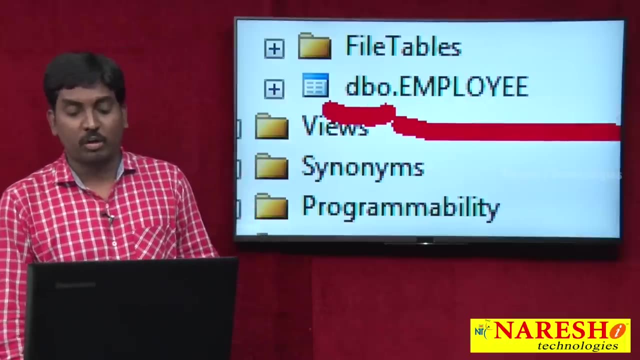 was there. it is called a user name. and what is the user name here? dbo, database object. So every table or view or synonym procedure function, Everything will be treated as a database object. So that was taken here. dbo username, dot employee. So after table was created, then what I want to do now, the next: immediately you have a 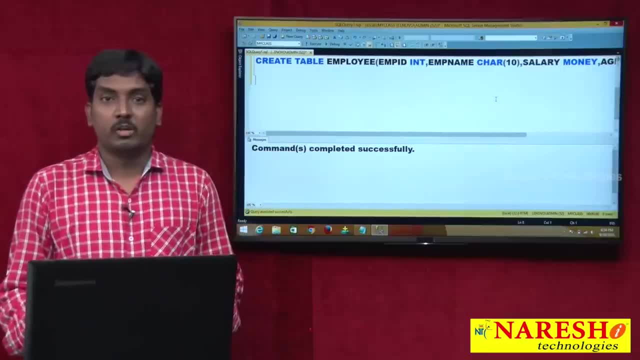 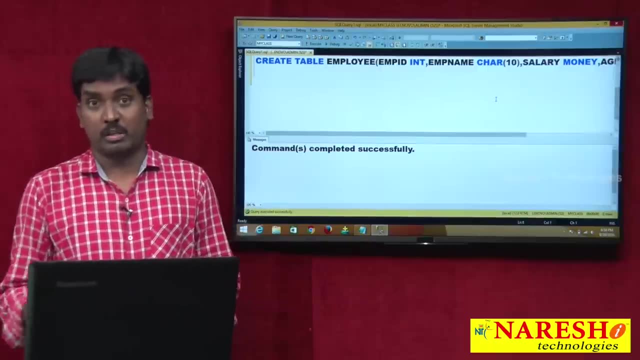 question: how to see my table structure. So that is immediately question you will be rise. So when I want to see my table structure, or structure of the table, then I am going to use- I am going to use one specific syntax whenever you want to view your structure of. 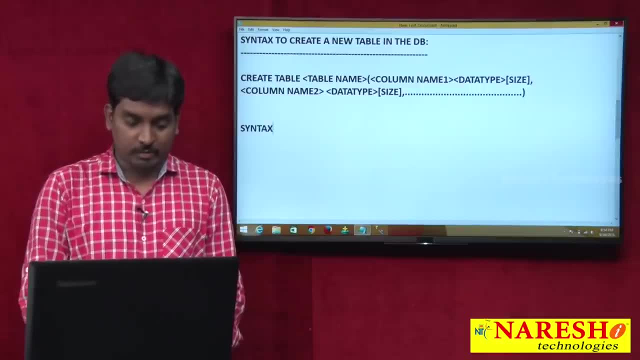 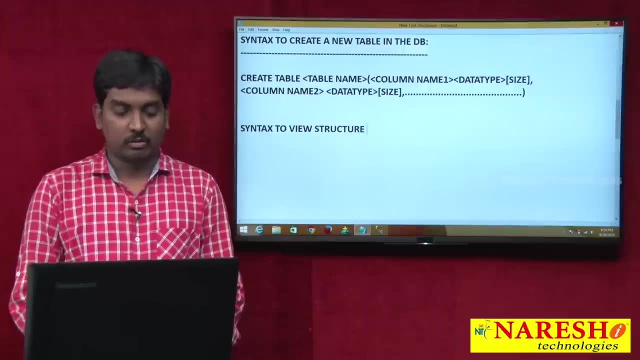 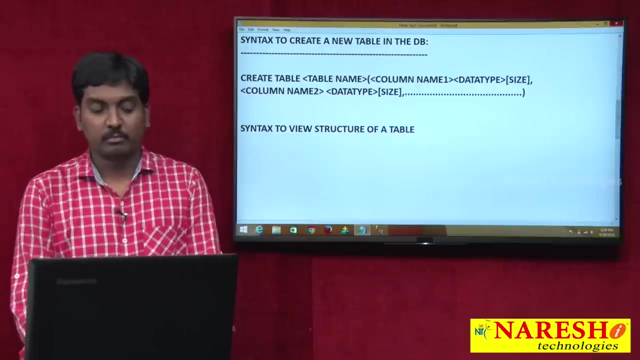 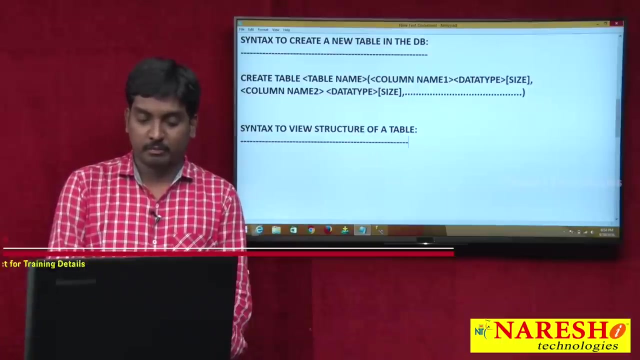 the table. So that we called as a so syntax to view, I can say now, I can say now the structure syntax to view the structure of a table, structure of a table. So now here, whenever I want to view the structure of table, whenever I want to view the structure, 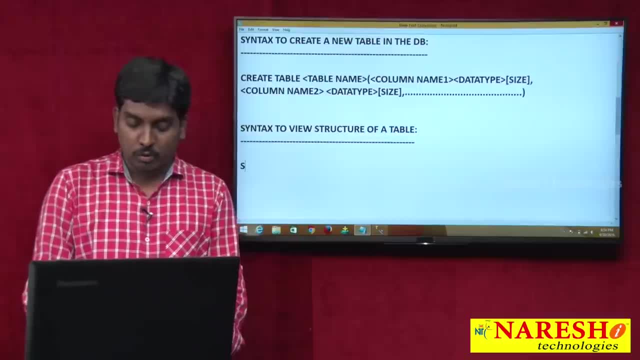 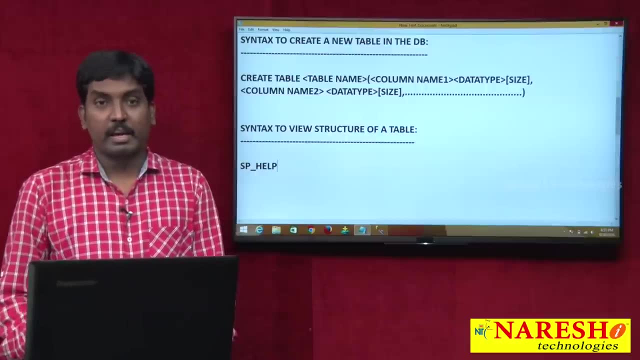 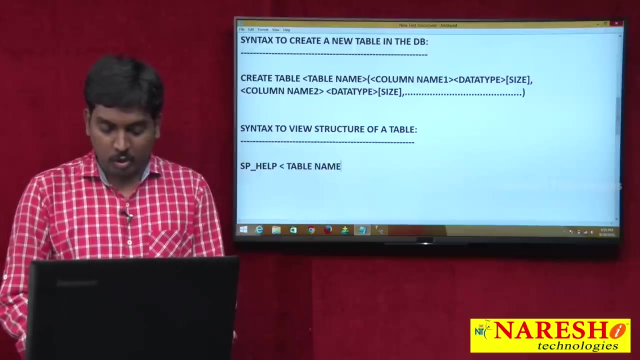 of table, Then I am going to using one stored procedure, The predefined stored procedure. I need that is called a sp underscore help, sp underscore help and later I want to send, later I want to send table name. ok, So what is sp underscore help? that we will discuss at the time of procedure, ok, concept. 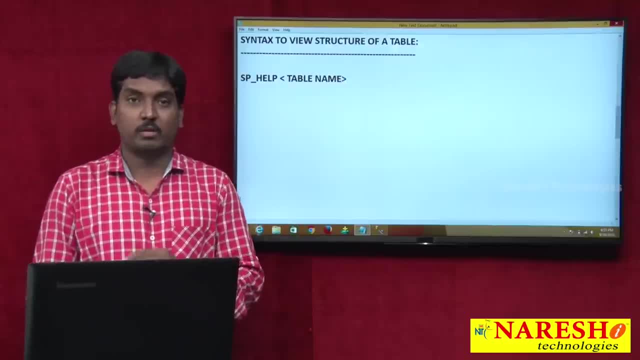 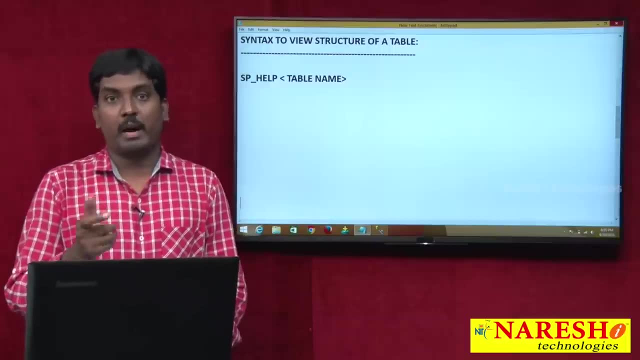 but here, simply remember, sp is nothing but stored procedure. It is a one of the predefined stored procedure in SQL server and through this procedure I am going to view my table, My structure of the table. So that is why here I was given my syntax was now sp underscore help. it is a predefined 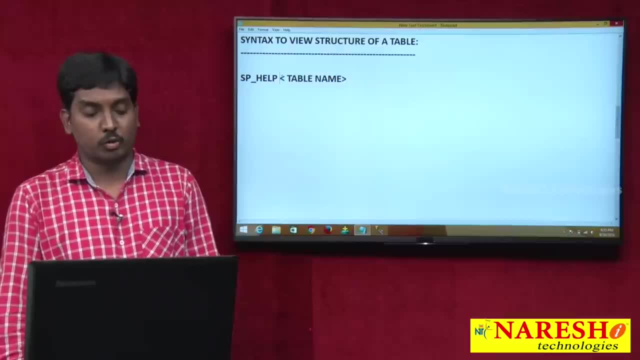 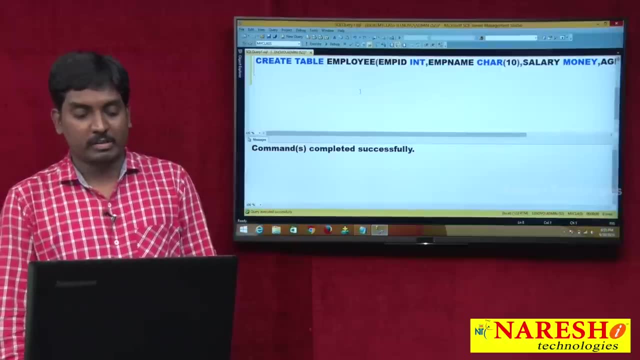 stored procedure and along with this predefined stored procedure, you should be send your table name. ok, So once I will send my table name, then I will be get my structure of the table. Now you can see, I just go to write my example. what is example here? sp. underscore. help my 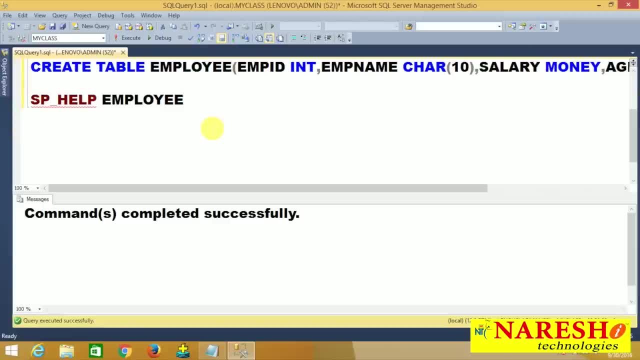 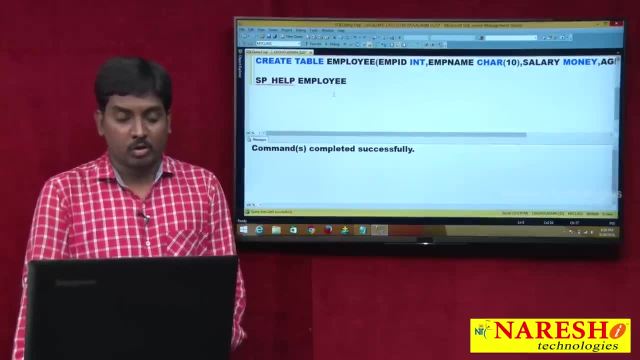 table name. what are the table name are you created just now? you just give it your employee, ok. After getting this, ok, now you are getting a red mark below, but it is not a error. ok, So why it will taking means in the same editor, why it was taking red mark means in the same. 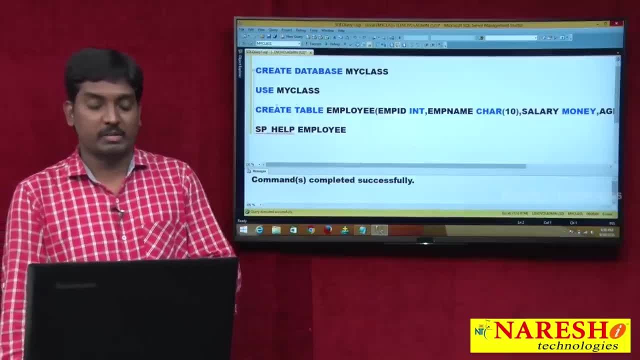 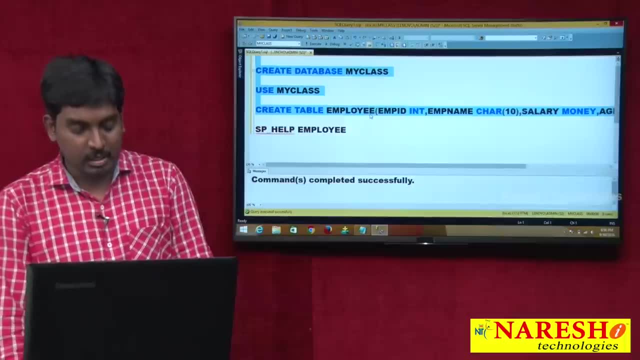 editor I am going to, or else I have some more statements here in this editor. So, for example, these statements, whatever it is there, that all statements I am going to just remove from my editor Once I remove from my editor. now, in this editor only we have a one query statement, that is. 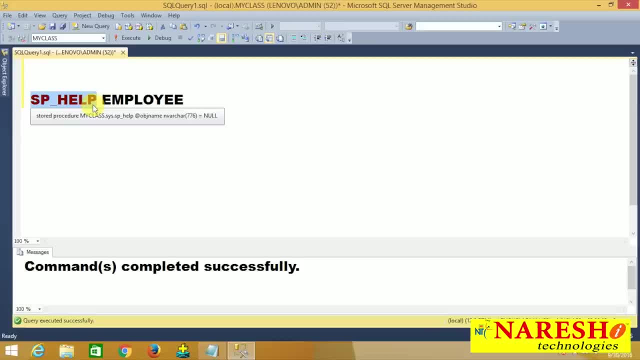 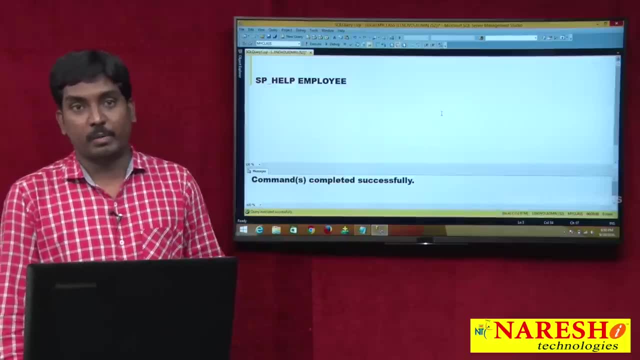 why time what it is happen, the red mark, whatever it is there, the previously the red mark is avoided. okay, because in the same editor if you have a more than one statements, then automatically it will take a red mark. but red mark. do not feel like it is a error. it is not a error. 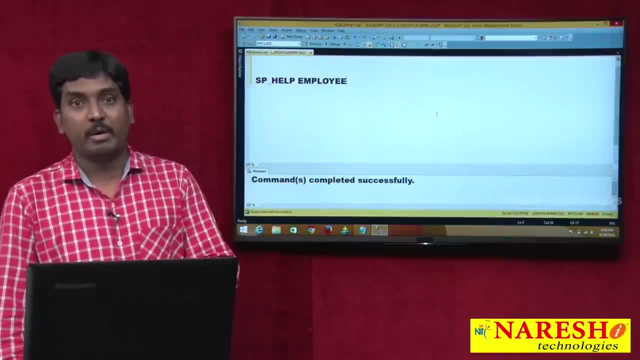 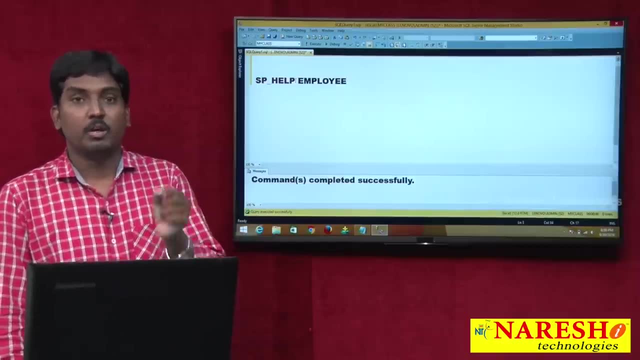 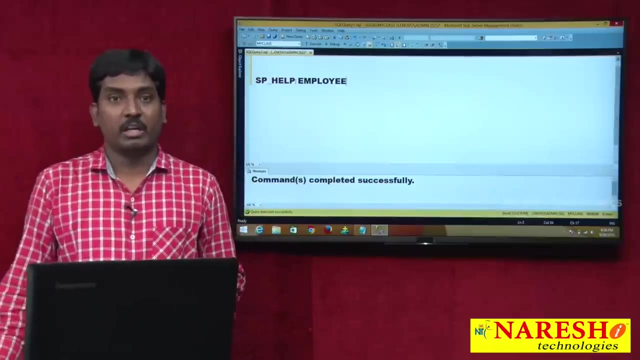 it just the representation is showing that in the same editor more than one statements are there. okay, So to avoid that red mark, you just avoid that all remaining statements and keep your necessary statement in this editor. then it does not show any red mark. color, okay, what line? what? whatever it is there that is avoided. So now I have at this red. 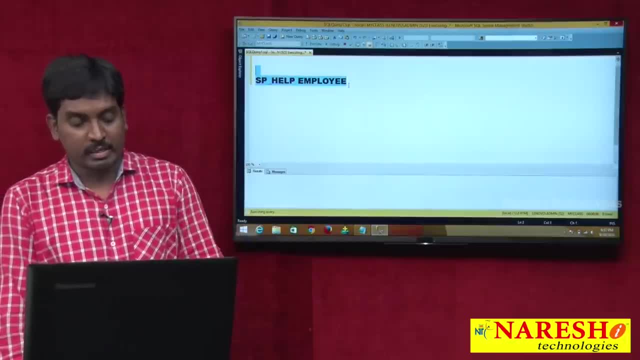 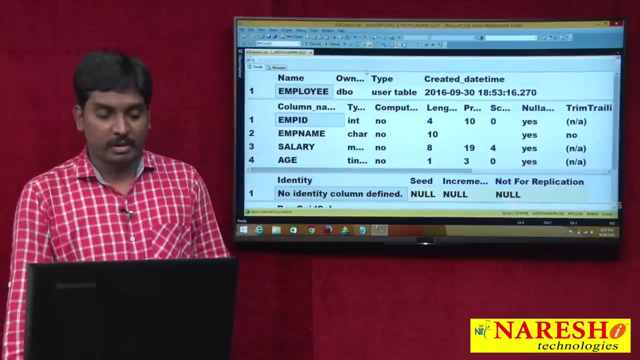 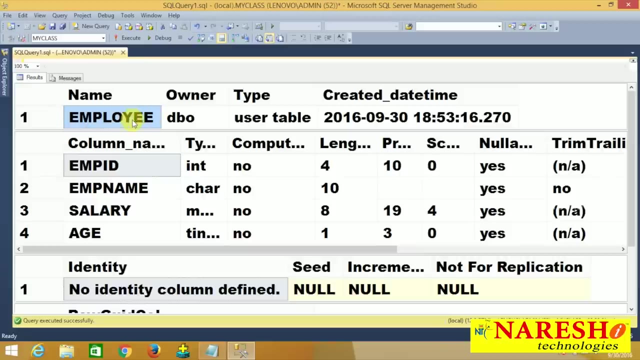 mark and later I just select this one and to executed. now, once executed, what is happened you can see. then complete: your table structure was displayed. The table structure was displayed here and you can see: this is my table name. okay, So on which table name? on which name I was created my table that was represented, name and this: 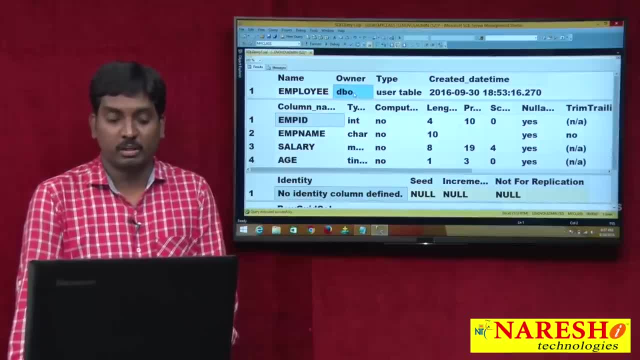 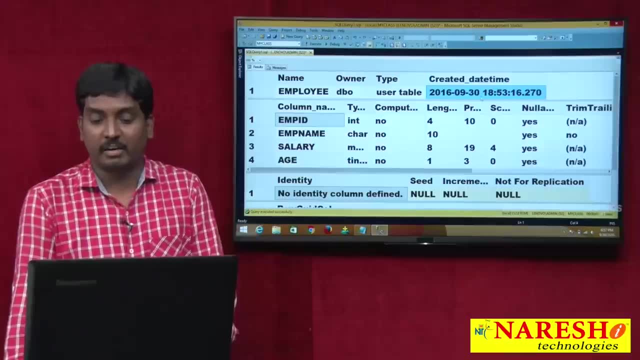 is owner db wrote. I said it is a user database object and this is it and I will show you. I will show you how to get my table name. So in this table is user table, because this table was created by user and this is the creation of date and 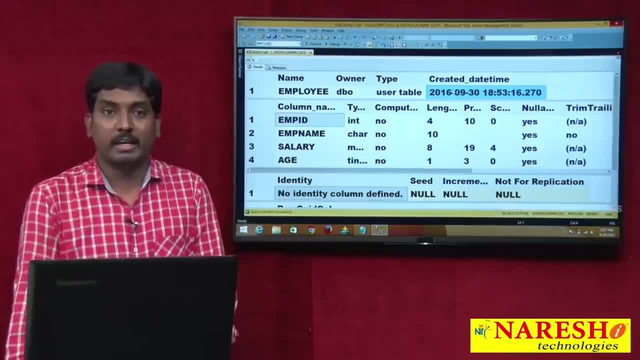 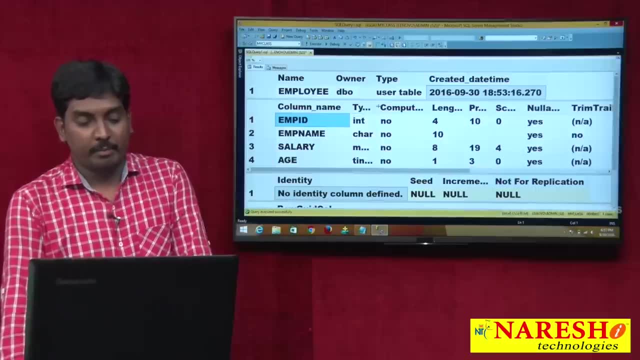 time? on which time, which date, are you created your table in the database that was showing here and later on in the next level. you can see. this is my column name and this is the type of the data type and computed columns, if any there. as of now, I did not create any. 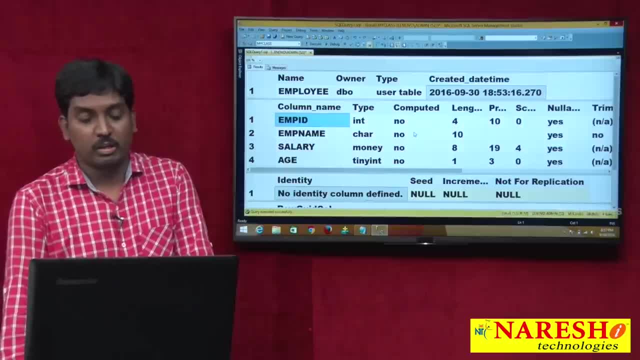 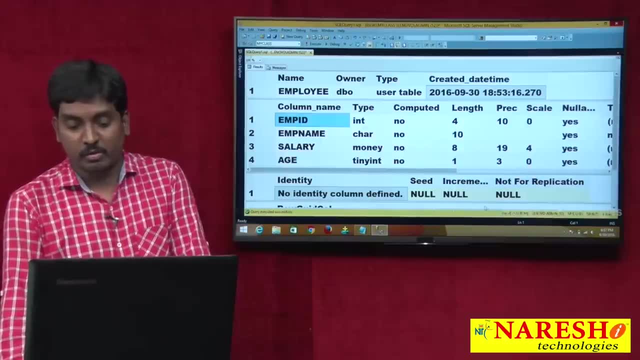 computed columns, but if it is there, it will showing yes, but it is no, there is no computed column. and later it is length, and this is precision and scale. so these are two values and finally, what it is here, the null bill. again. next, what it is here: null bill, column. 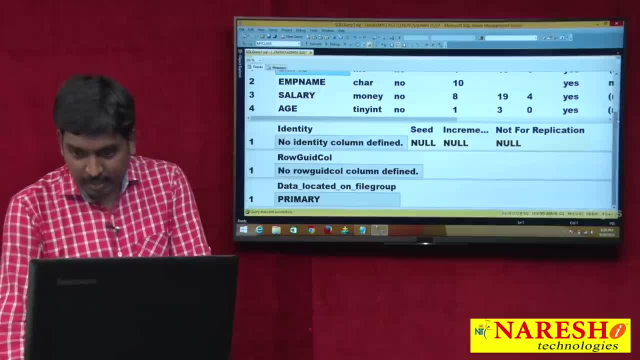 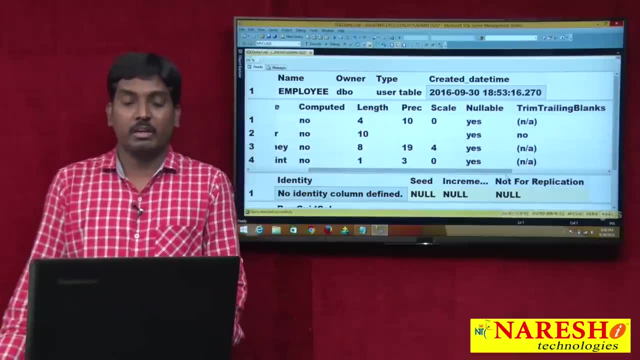 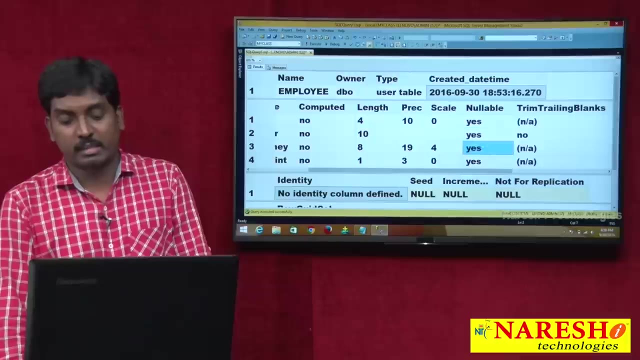 was there here, this null bill. you can see now this is my null bill. So null bill, column and later null bill, means, you know, every column by default accepted null value. that is why each and every column, the four columns, whatever I created in the table so that all columns are accepting S, S, S and S. 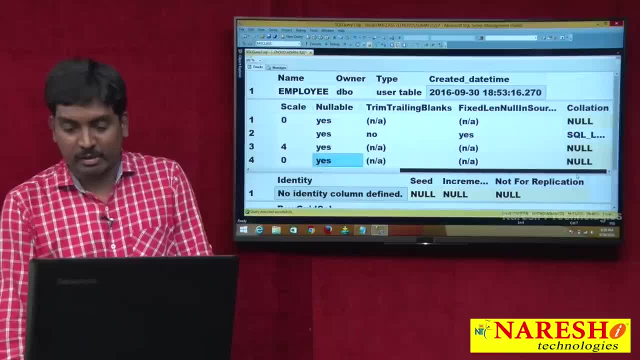 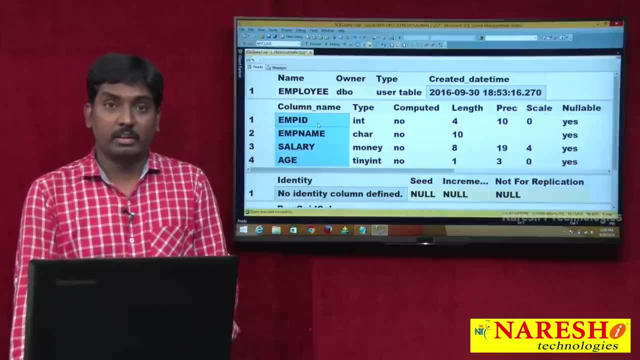 And later I used here: trim ok the fixed length. these are not necessary. you just avoid this, ok, so now up to here. what is now? column names? are there the column names, whatever the names I was given there at the time of creation, that all names are showing now? 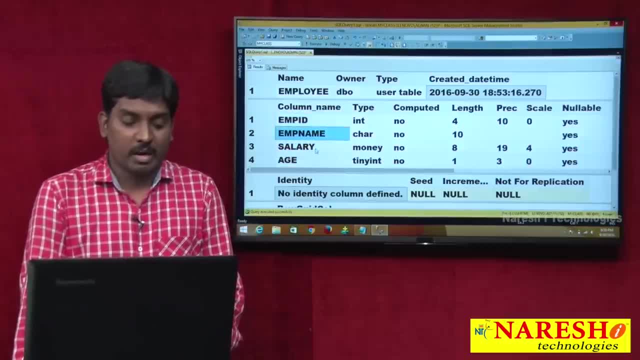 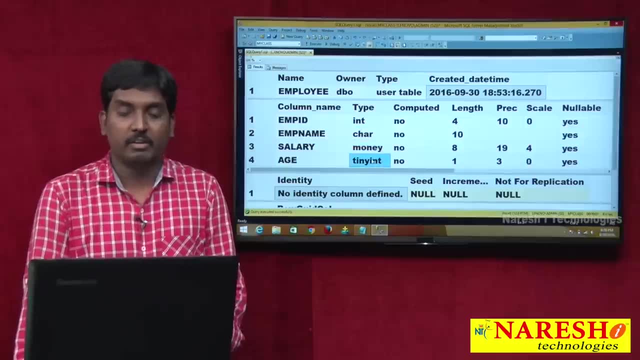 So one is first, one is what now? EMP ID, EMP name, salary, age, ok, and later I was given the type of ok column: integer, type, character, money and tenant. Later, there is no computed columns, the. what is the computed? we will see in the later session. 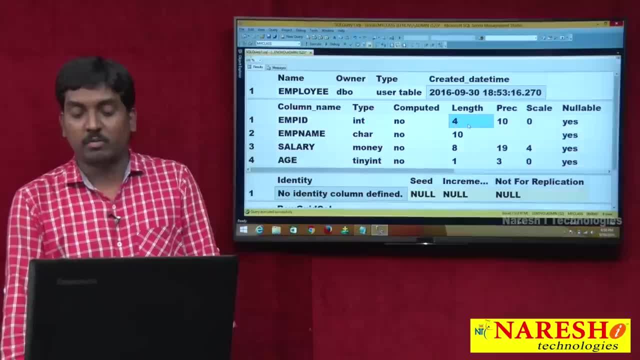 later, length was there. so tinny int, tinny int, the length is what? now 4 bytes in the same, to same character. I was given here 10 bytes of memory and money. if I use money it will take by default 8 bytes of length and tinny int will occupy 8 bytes of memory. ok, and this. 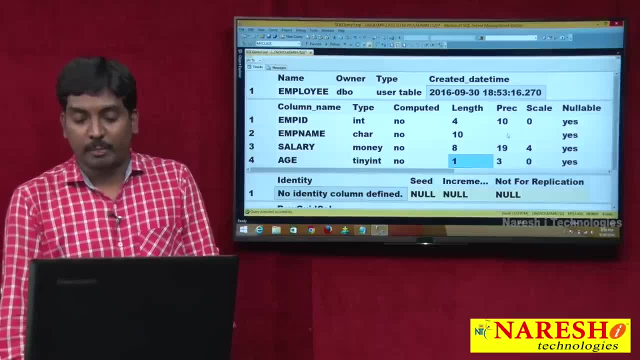 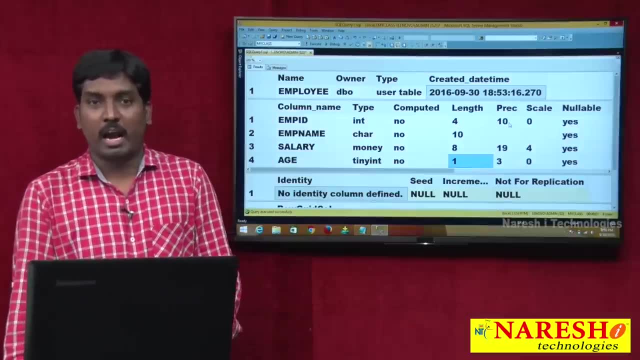 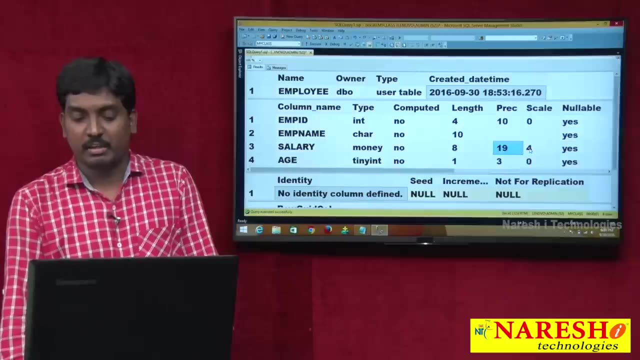 is what it is here. precision values: ok. So, and precision, when I take 4, precision is 10, ok, and the precision is nothing but simple. I can say range, simple, you can identify it is a like a range, ok. And now Here money was. range was 19 comma 4. this is precision and scale: ok, the money data was: 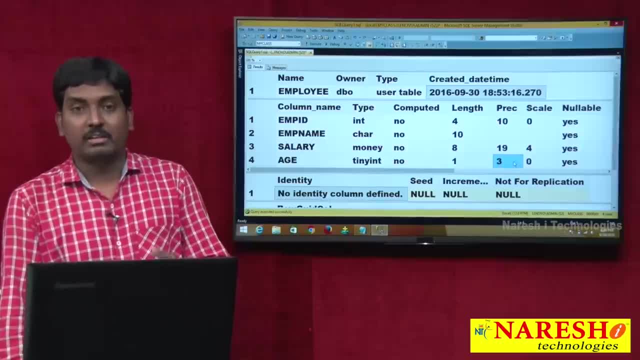 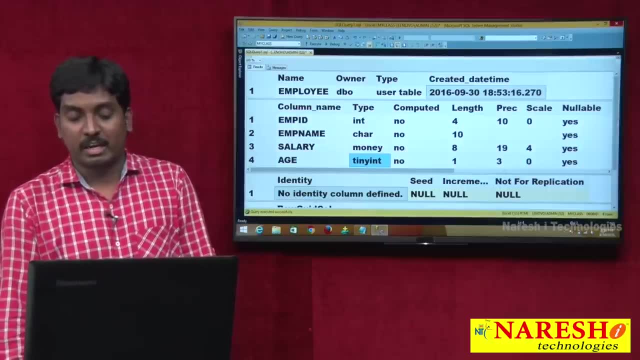 given, and this is tinny int range. is what now? 3, 3 means 3 digits, so that means actually tinny int range. what is now 0 to 255? so that is the range, the range 255. it was represent 3 digits, ok. 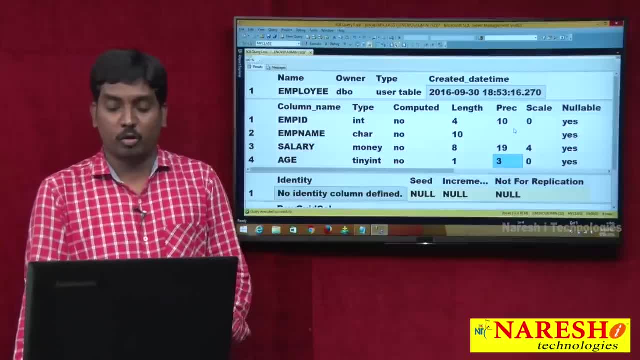 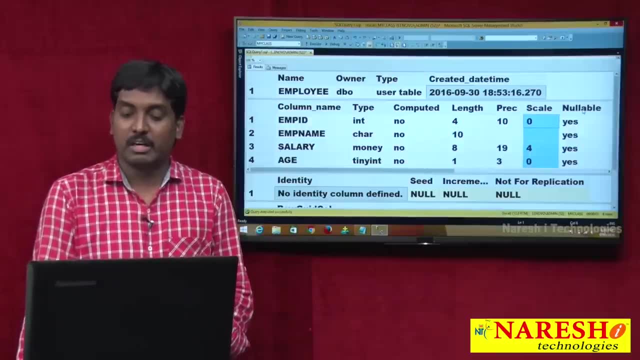 So now this is the precision. you just remember it is a range. ok, So now scale was there. but what is scale? we will later we will discuss, and this is what it is here: the type, length, precision and scale. and nullable means every column is accepted nulls. that is why it was showing SSS. ok, 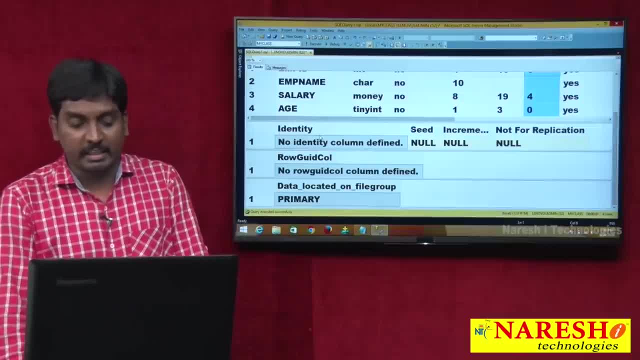 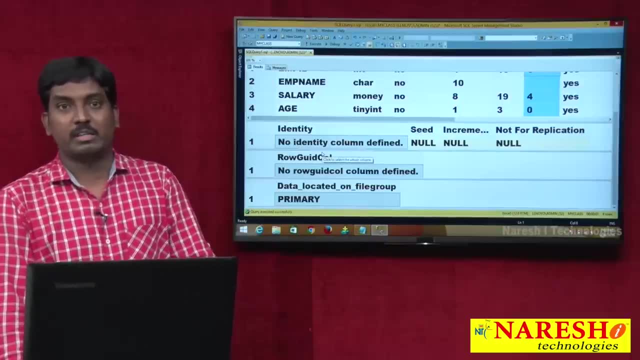 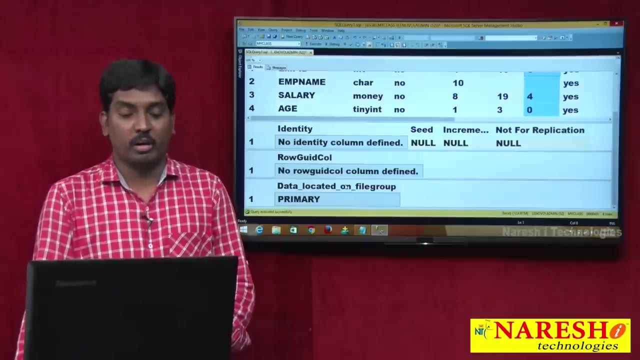 And later on, later on the table. I did not create any identity, any row, grid and any primary or foreign keys. this kind of constants I did not apply on this table. this is my first sample table. I was created without having any other facilities. ok, So that is why everything was showing here. no, no, no, ok, so now this is the way to view. 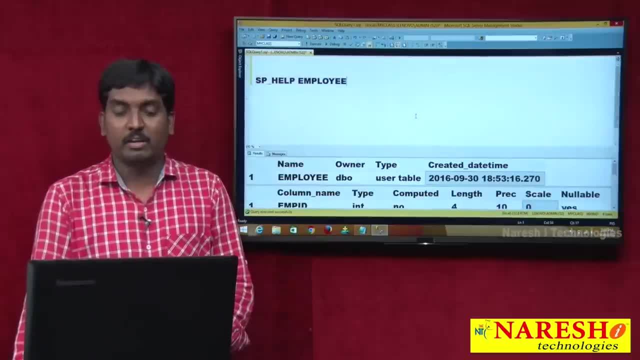 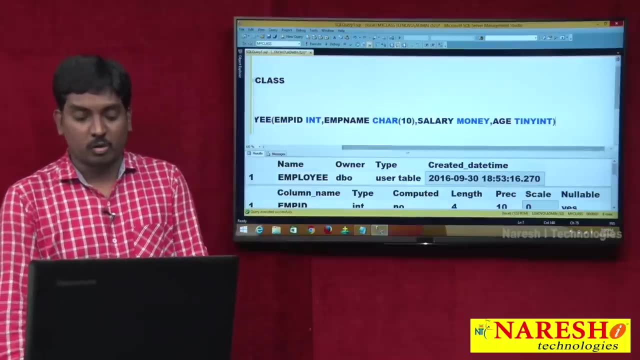 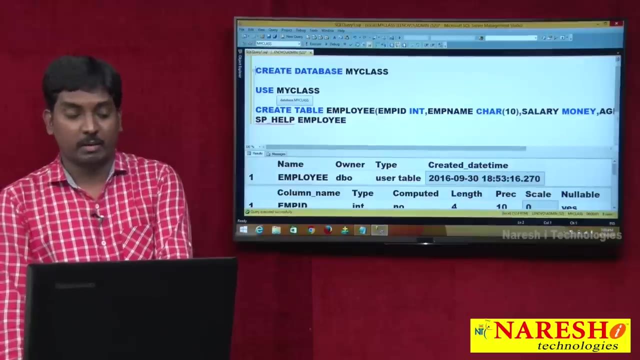 your structure of the table. Ok, after design your table, you just go to call like this: then you will be finding your complete structure of the table. ok, So now what is happened here? in this? I just created one database first. you want to create your database first of all, and later select that database and after that you can create. 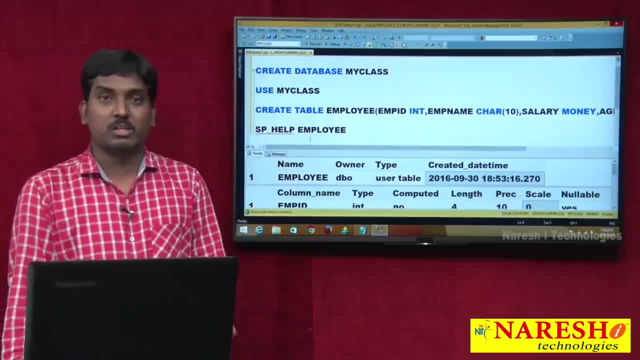 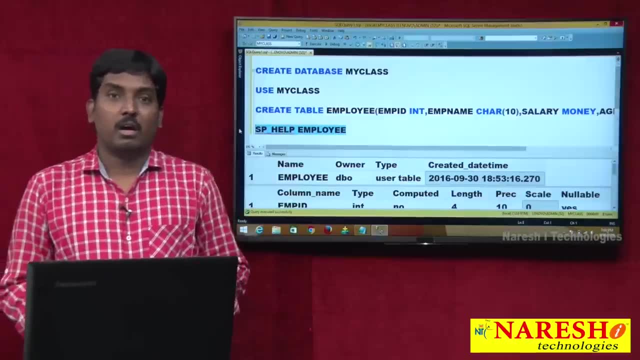 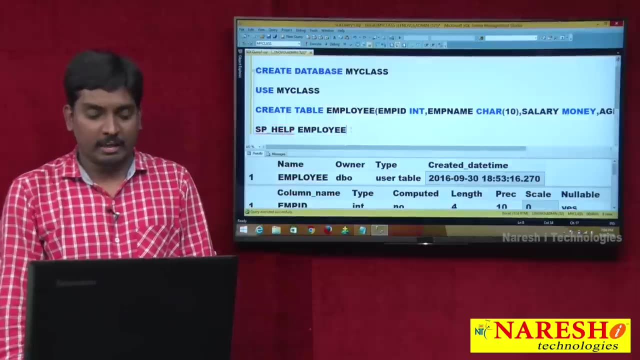 your new table. after creation of new table: if you want to view the structure of the table, then you can use this SP underscore help: table name. ok, so this is what now create command: how to use And how to, How to work. ok, So now the creation of table and database. we discuss here and later here observed when 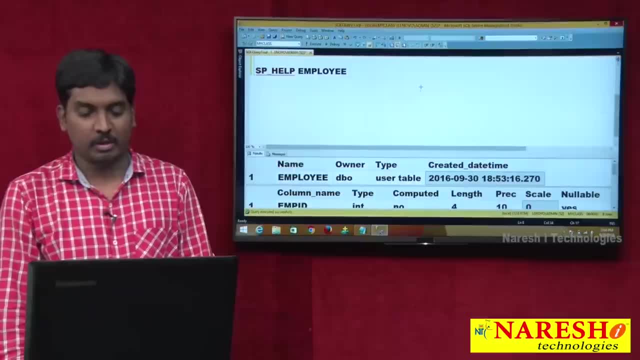 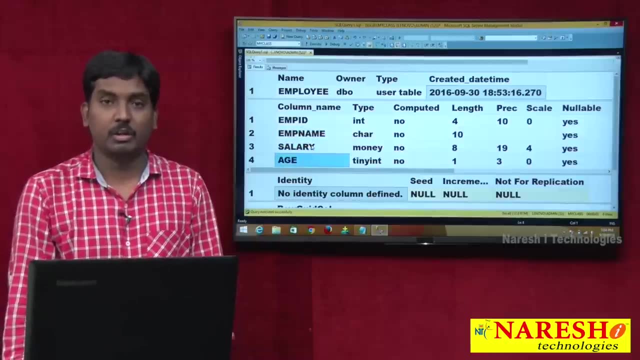 I was created my table. ok, can you see the structure of the table now? ok, in especially, you just come out here the structure of the table: EMP ID, name, salary and age. ok, So now after design, or after create your table structure, if you want to see graphically, you 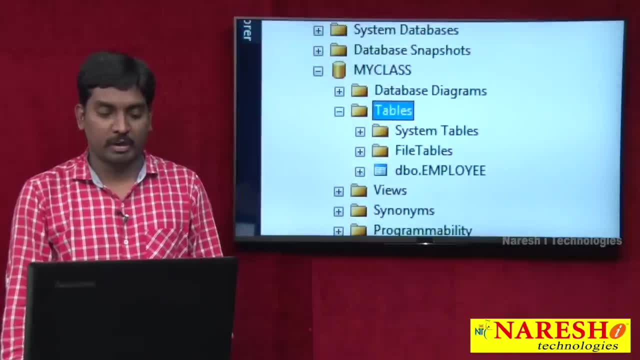 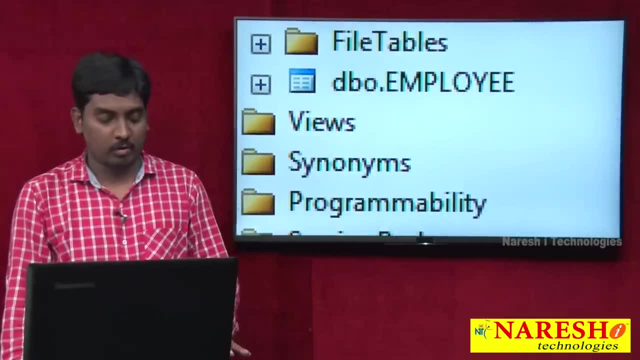 just come out here object explorer window and go to your required database- my class and later- you just go to table and after going to table folder, now your table was showing now and this table was having some addition symbol. was there here? addition symbol is nothing but plus symbol. 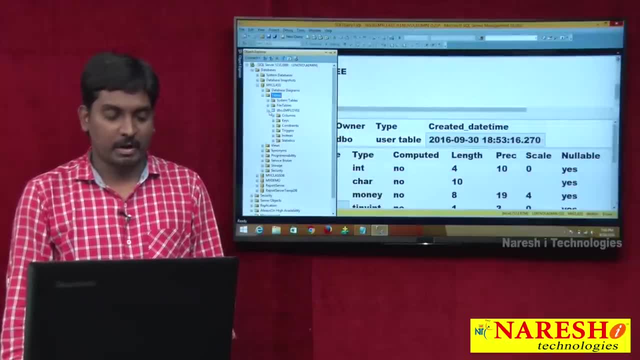 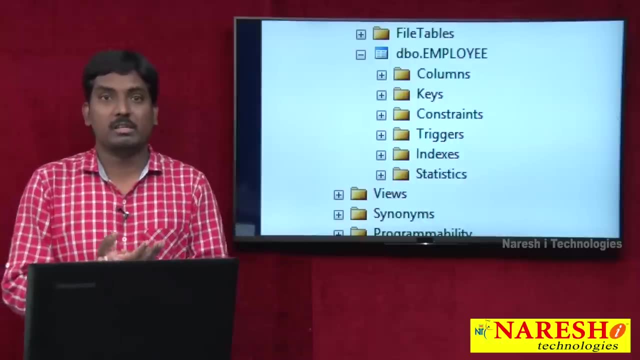 So this symbol you just expand here once. I want to expand here, ok, on the table, expand here on the table. what kind of the things or facilities I can apply on a table that each and every facility information was going to store in a particular folder, for example? 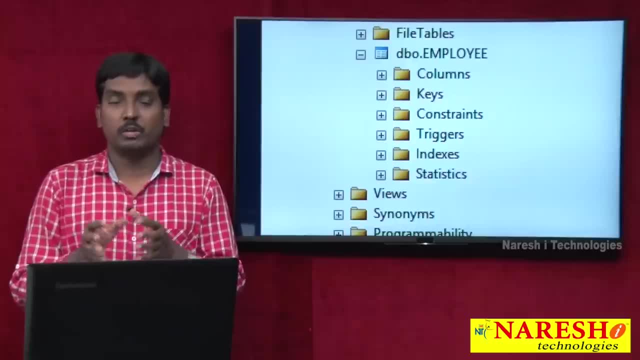 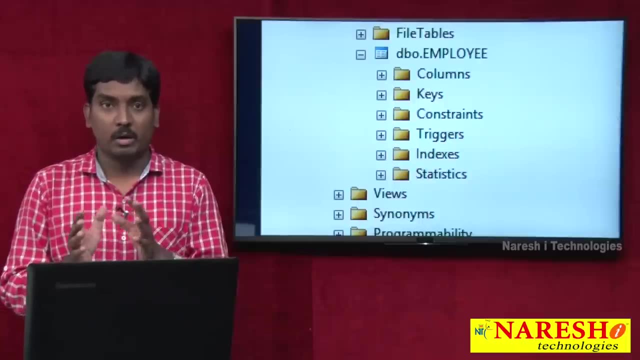 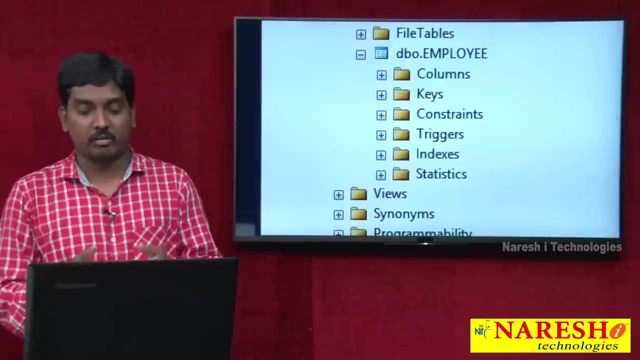 columns are there. So in columns folder what it is storing, your table columns information was storing ok and later keys like a unique key, primary key, this kind of keys. if you applied on a column of a table then you can use the keys of storing under this keys folder like a constants triggers. 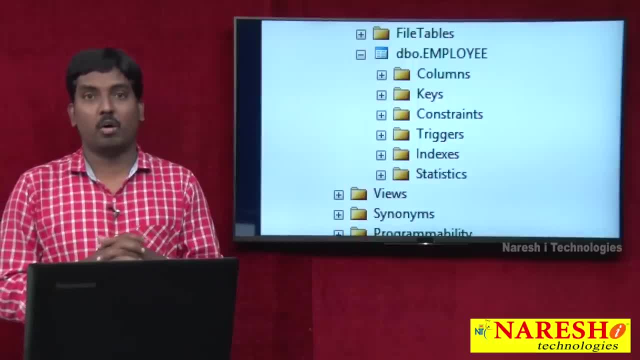 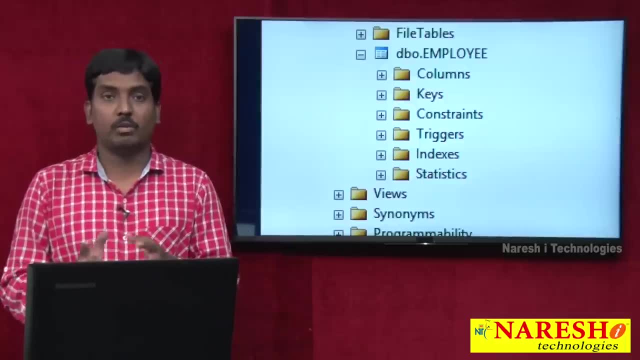 indexes and statistics. So which you applied on a table, those related information was going to store in the related folders, For example, best example. I am showing now. so, as of now, what I did here, I just created my table. So I just created my table with some columns, that is it, and column name: data type: I was 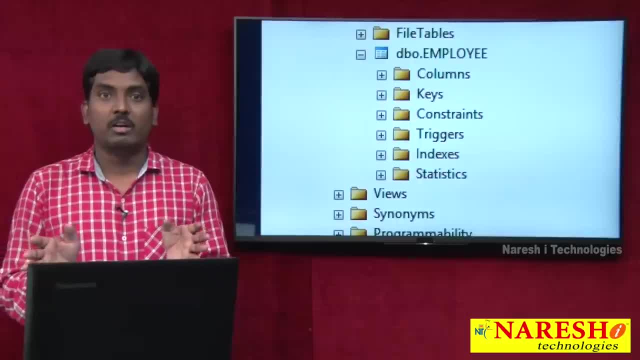 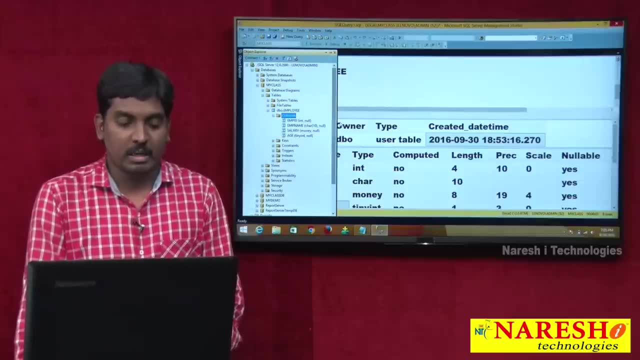 given. but other than this, I did not apply any other special facilities on this table. ok, So that is why what it is happening here. once I want to open this columns folder, then you can see the. what kind of columns are you given at the time of, at the time of designing? 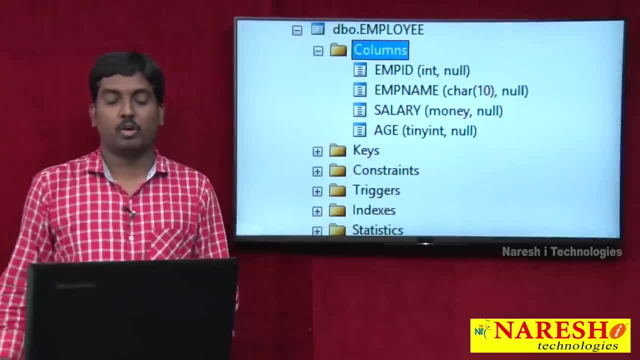 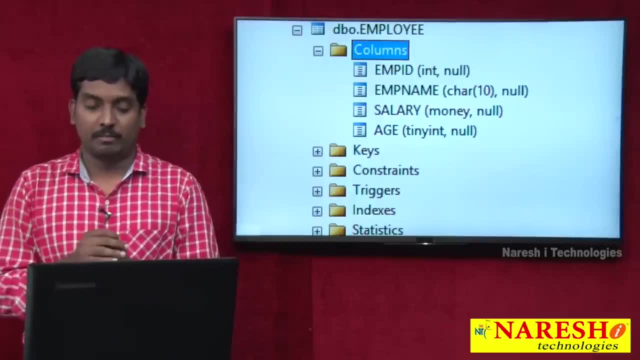 level. those all column names are showing now. ok, So it was showing you are. you can see clearly. EMP ID NT is a data type and by default your column is accepted null. In the same to same EMP name, character data type of 10. the size was given 10 and null. 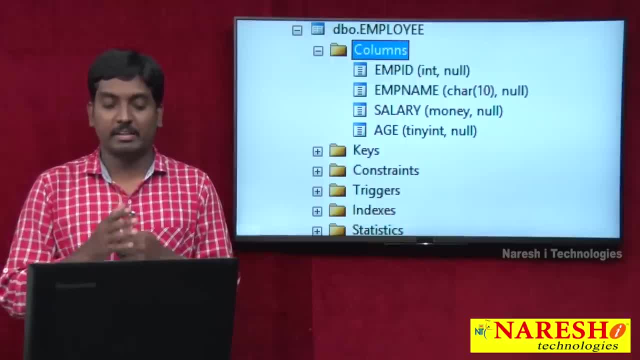 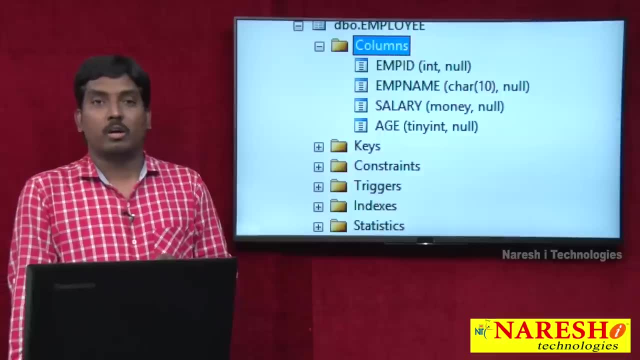 is accepted. salary money: null is accepted. age tini: int. null is accepted. That means so how we observed and how we viewed your structure of the table. ok, by using sp underscore help command. ok here also, same to same. you just come to your object explorer. 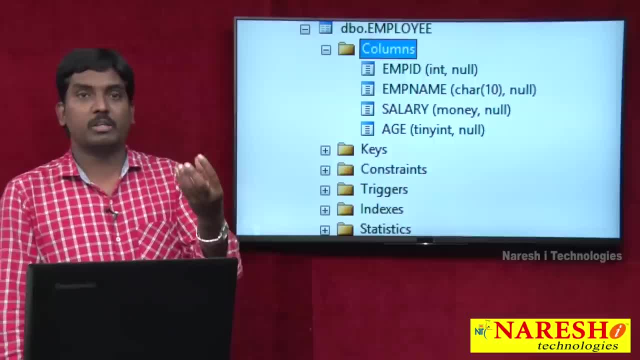 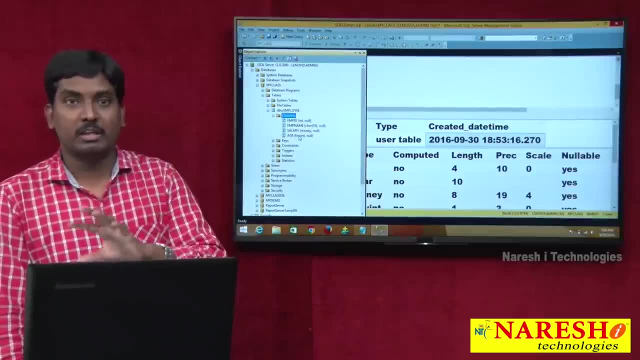 and go to your table and open your columns folder that all columns details was holding and storing here. So now in that way also, you can see your table structure, which columns are there, which data types applied, what kind of names I was given to my columns. ok, this all kind of information. 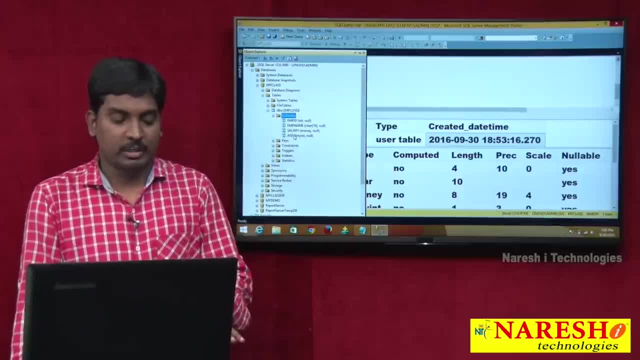 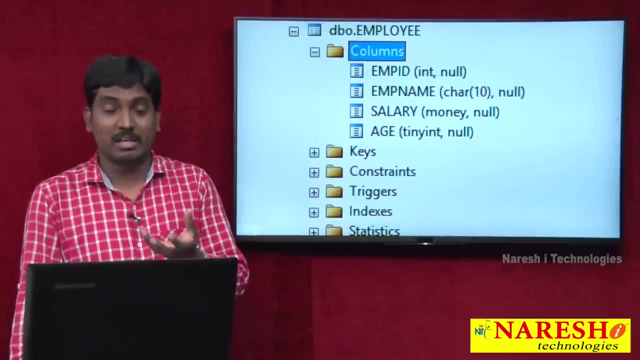 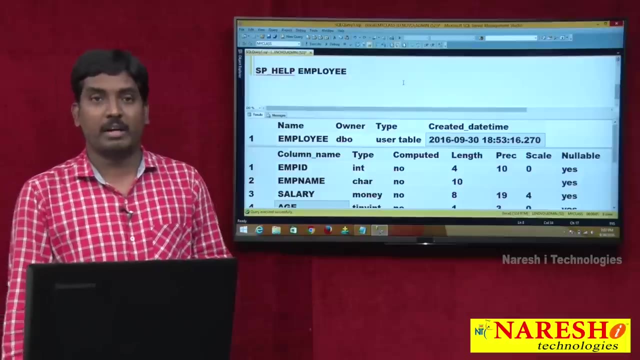 you can also. you can see by using this: ok, this object explorer window without writing my query sp underscore. help: the query is not required to view my table structure. this is graphical, I can say graphical. you can view this structure of the table. So, after table was designed, created in my database. 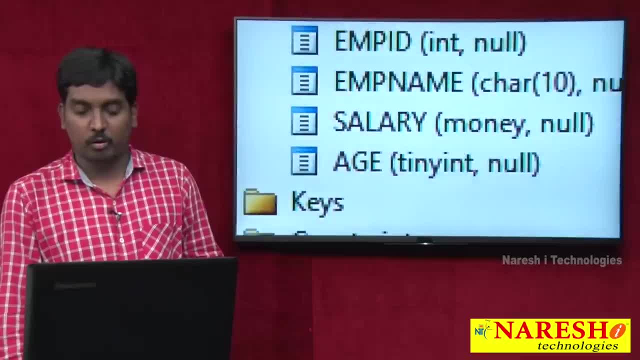 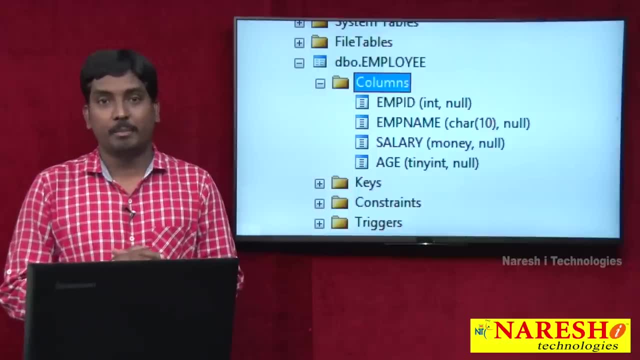 Now what I want to do. I want to modify, I want to modify the table structure. the what kind of modifications I can perform on my structure of the table means ok. So, for example, you observe, for example, what I want to do now. for example, initially, my 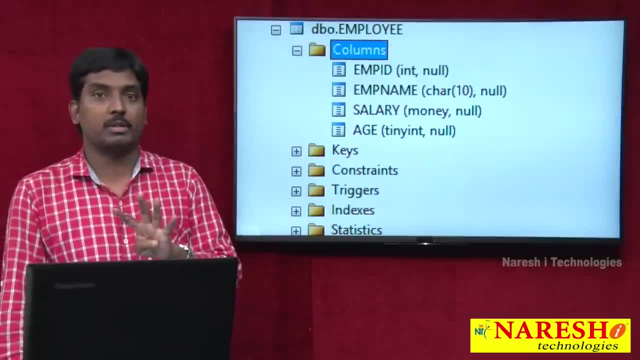 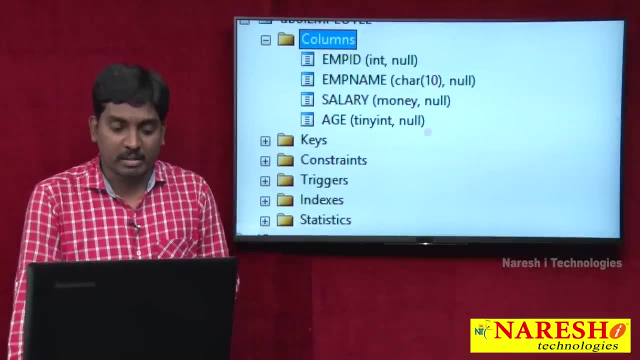 table was ok, created with how many columns here? 4 columns, ok, 4 columns we created at the time of table creation. But in this, in this, if I want to change, for example, first one option, I am saying that, for example, how do you identify EMP name was there. 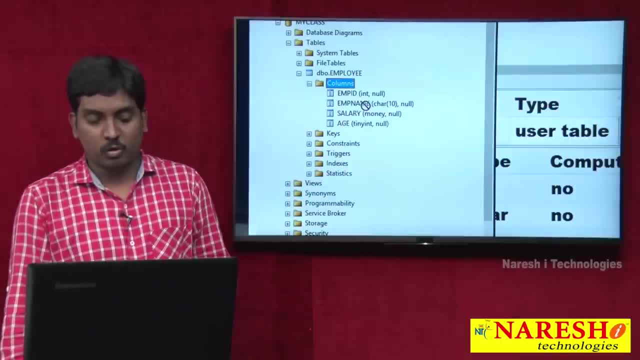 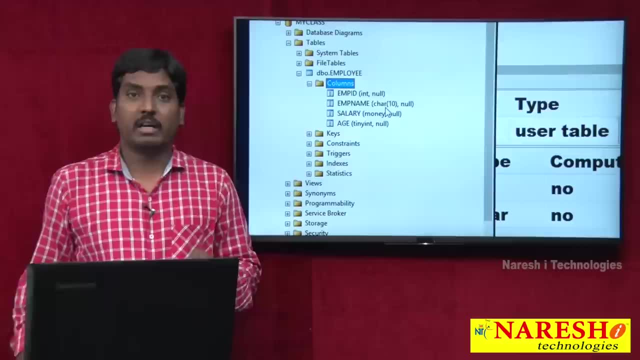 This column was there now. So EMP name column. so this column, data type I was given char of size. of size is how much? now 10.. But char data type: it is a fixed length data type, so that means how much size are you assigned? 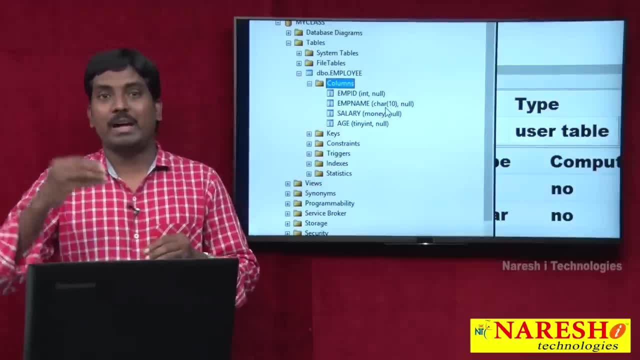 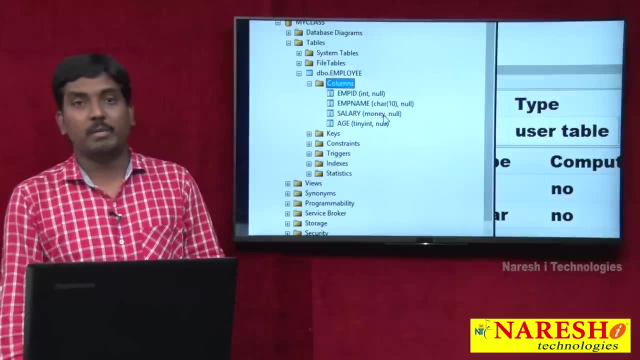 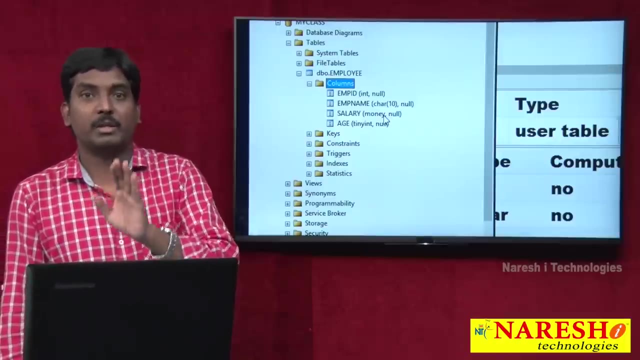 to the column, along with your char data type, that many bytes are allocated. ok, So that means, for example, char of 10 I was given now. So 10 means maximum. into this column maximum i can send my characters up to 10 characters expressions. 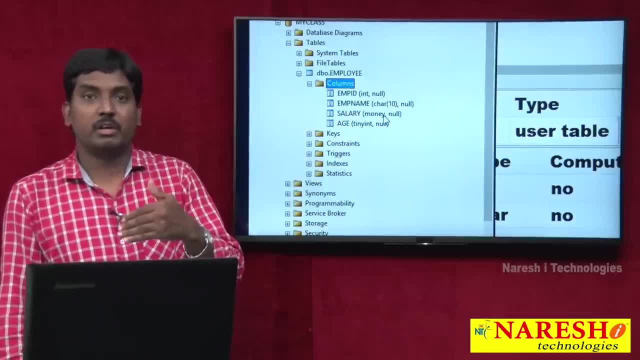 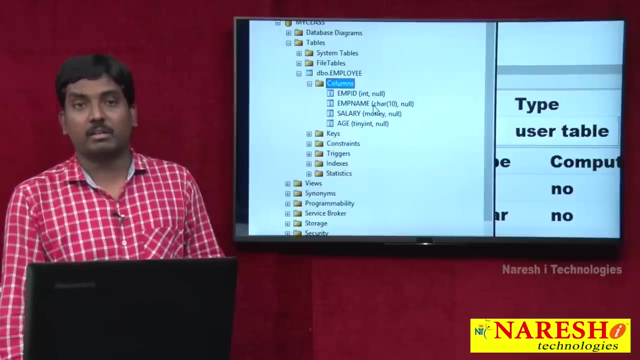 only i can send. but the 11th character expression if i want to send into this column, it is not accepted. why? because your length is how much? now, 10 was given, so that means 10 characters will accept it. okay, because each character will take a one byte memory. okay, and later, character car i. 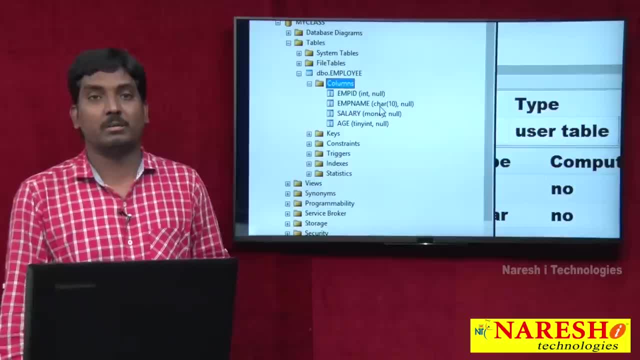 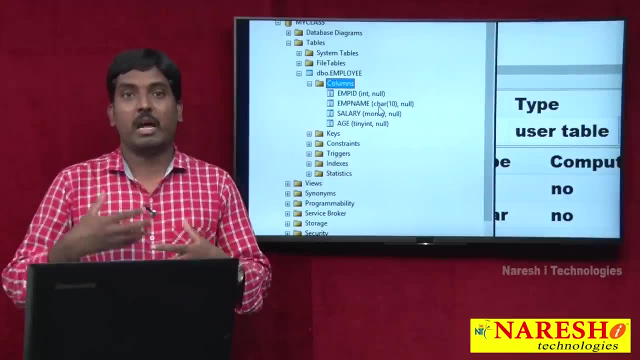 was given. cat data type is a fixed length data type. it is nothing but static data type. so you know, if it is a static data type, what is the problem? memory is problem. okay, unnecessarily i am going to wasting my memory. so that means what i do here and what i am doing here. so first of all, 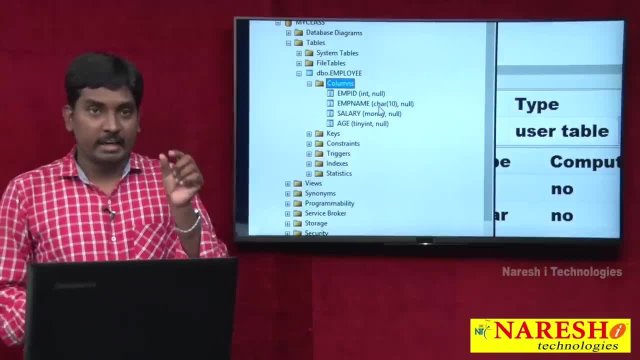 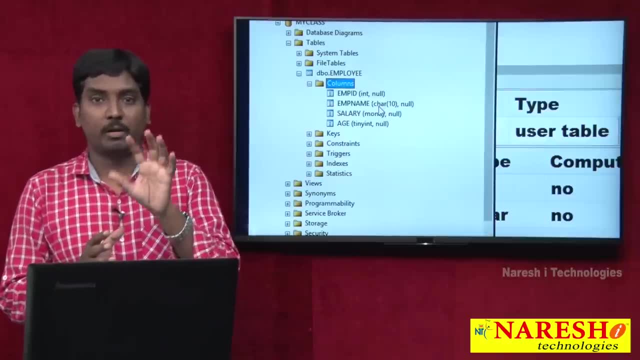 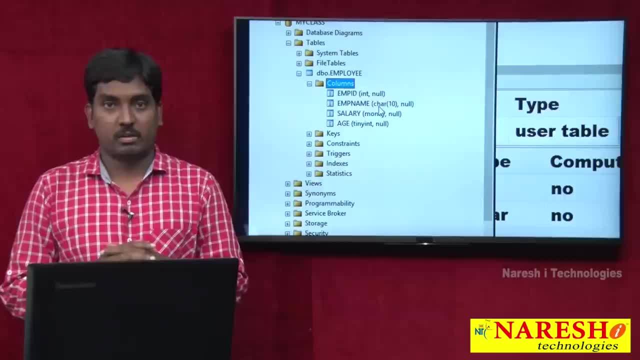 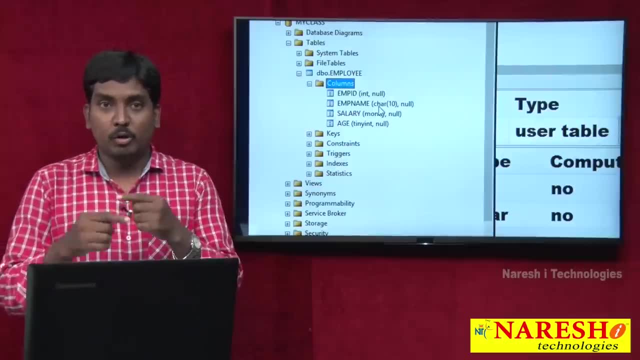 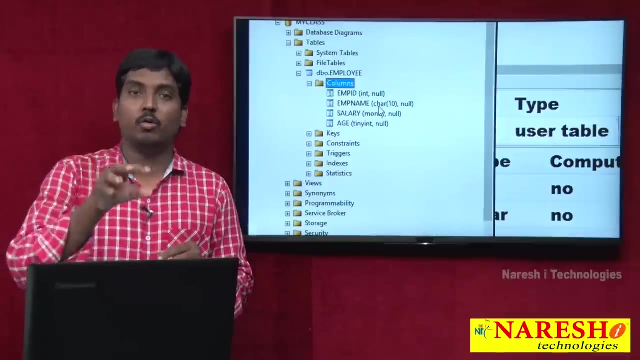 for example, initially my table was created four columns for after some time. assume like this this employee department name i want to add. so i am going to adding one more new column to my adjusting table. already table was created on that table. i want to add a new column, but how to add a new? 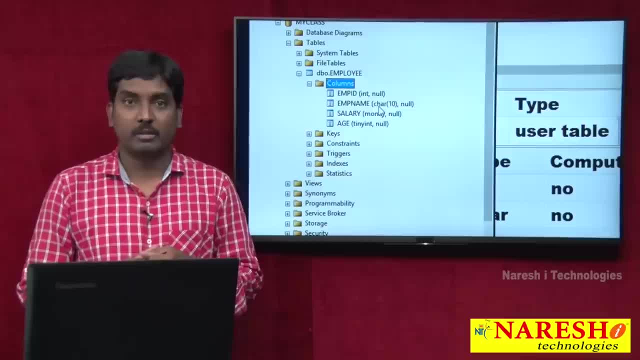 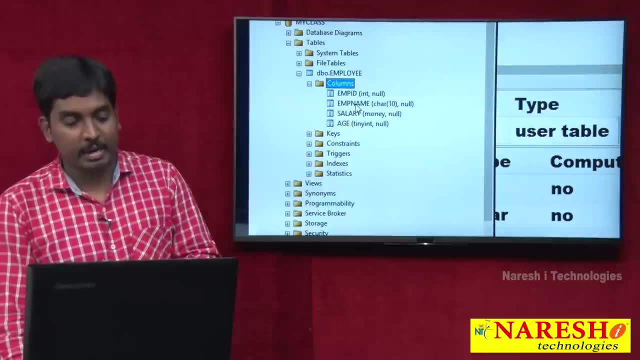 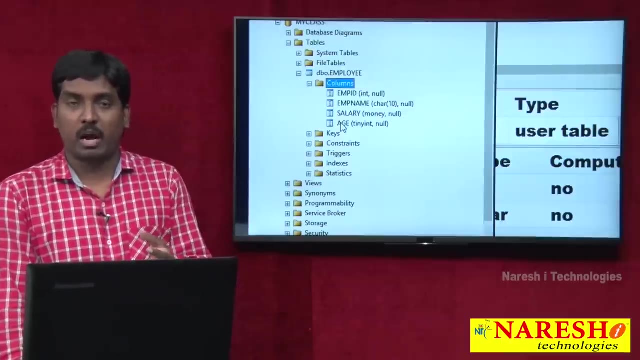 column to my adjusting table. that is second operation. third operation, what it is here, for example, initially my column names. i was given emp id in name, salary age For any column name. do you want to change? I do not wanted this. column names. I am going to change my column name then how we can change. ok. 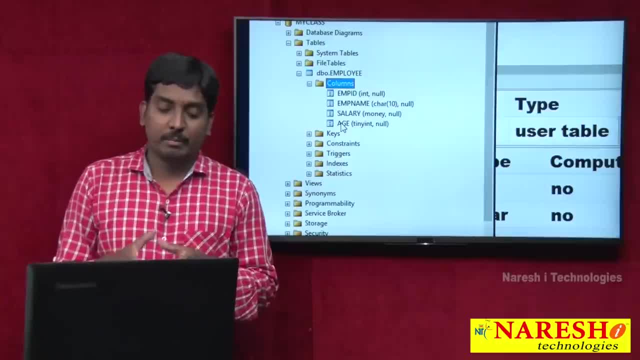 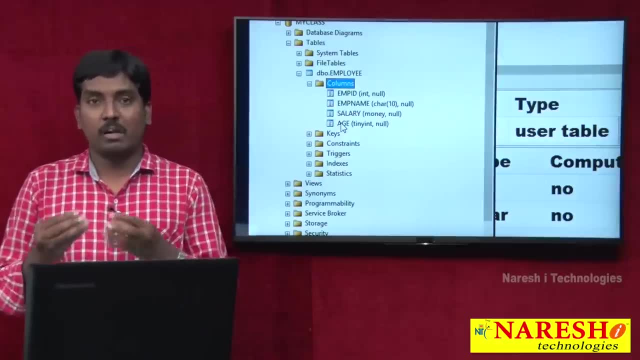 And later, last one, the last operation, what it is here, For example, in this 4 columns assume, like this age column is not required for me. So I treated this as a unwanted column which is not necessary to me as per my requirement. So at the time, what it is happened here. 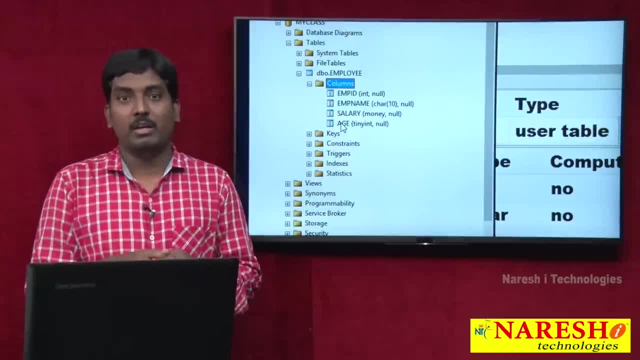 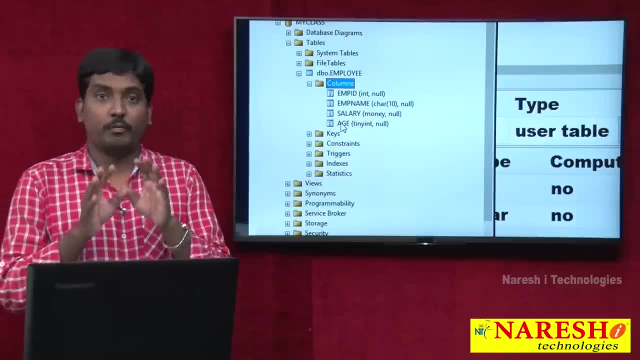 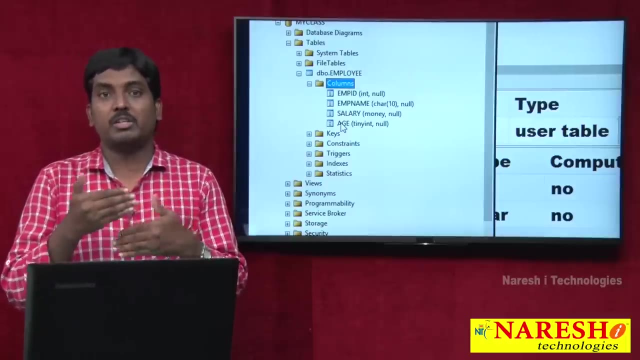 how many columns are there unwanted columns? are there in the table? those unwanted columns you just remove, yes or no, But how we can remove. ok, So these are what it is: a 4 operations you can perform on your adjusting table structure. That means the modifications I am going to. 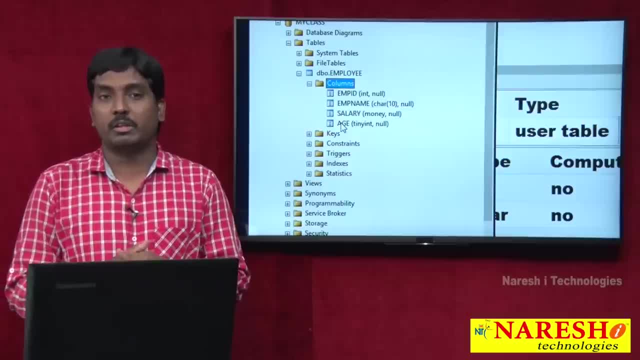 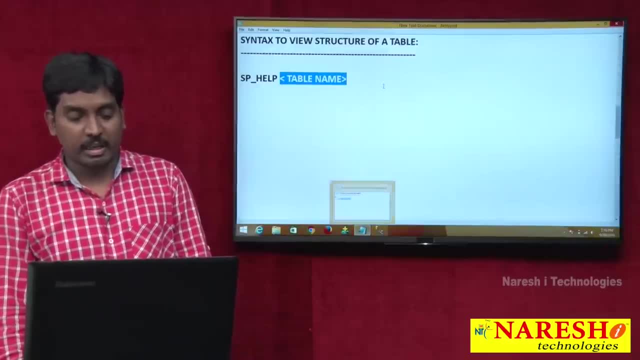 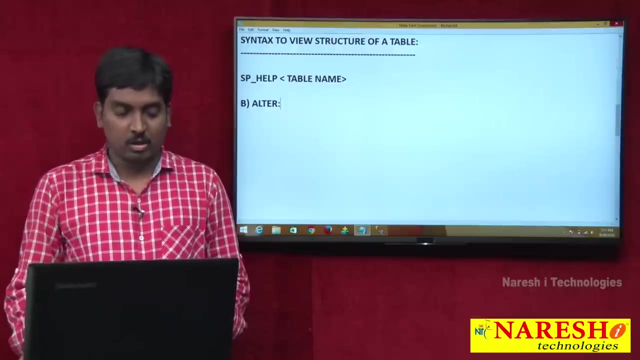 doing the modifications I am going to doing on structure of the table. But if I want to do this kind of modifications, then which command I need? if have it means, then I need the next command. The next command is what? now My second command we called as a. which command here Altered? 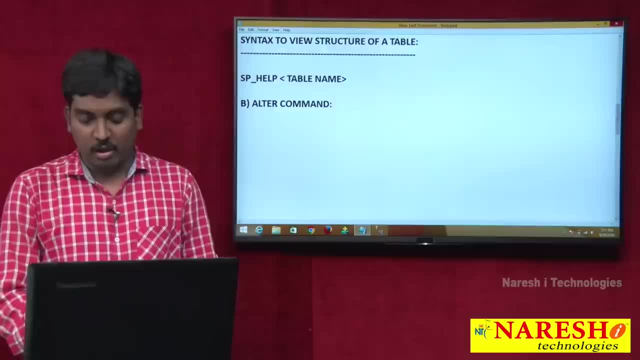 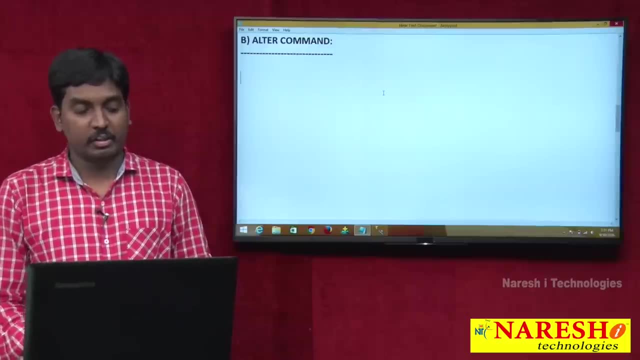 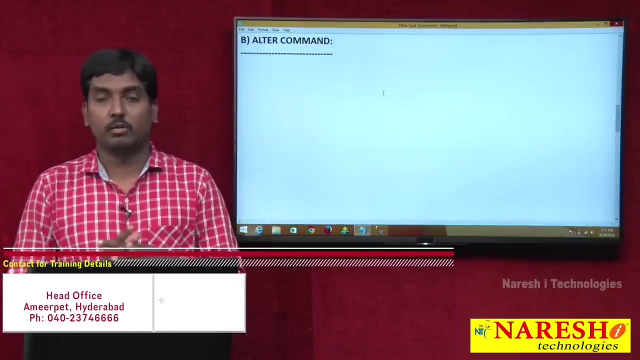 So alter command I am going to taking now, ok, So if I want to do the modification, ok, or changes, ok, any modification or any changes we want to perform on structure of the table and also structure of the database, also I can use this alter command. ok, So, 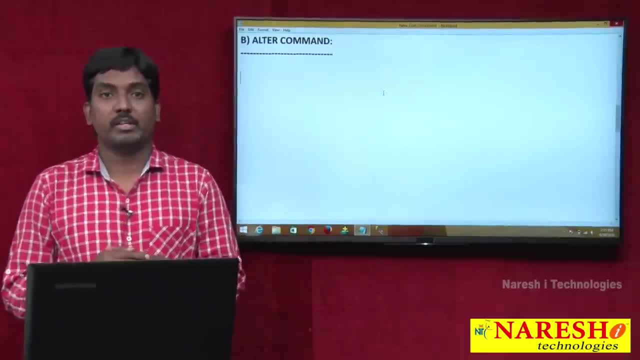 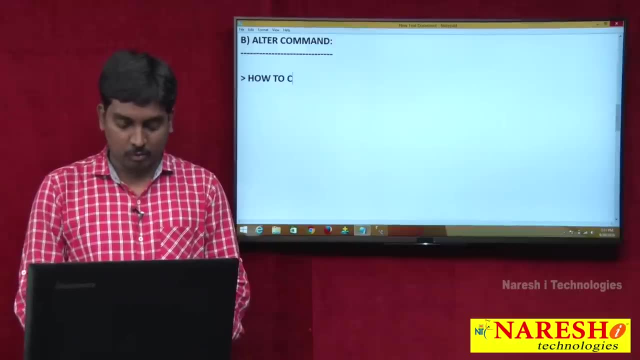 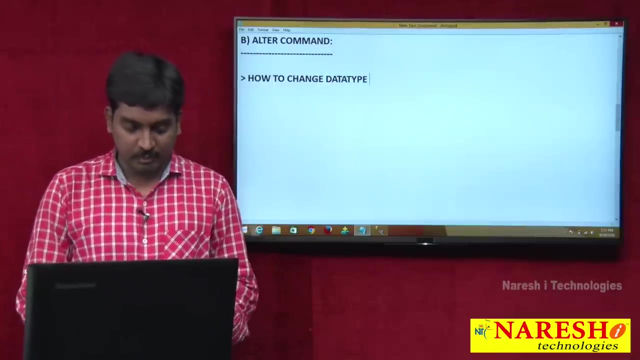 this by using this alter command, the what kind of modifications I am going to perform, The modifications I can do it on my table structure means: just now I said my first one. what I said here, how to, how to change, So how to change data type and also and 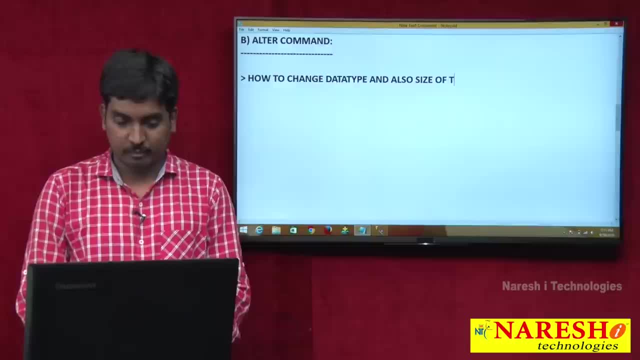 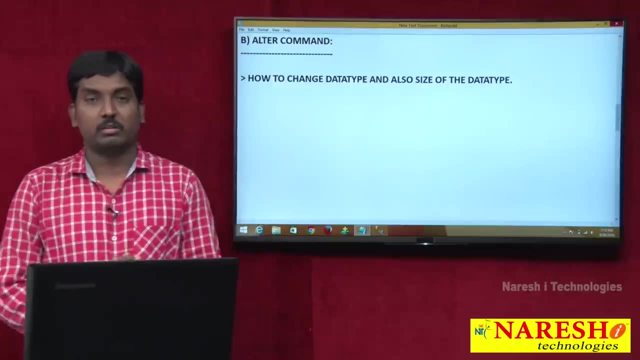 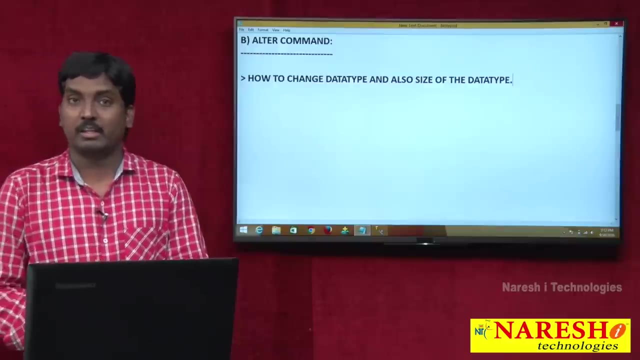 also size of the data type. size of the data type. ok, So now I can- how to change- This is my first operation on my adjusting table, So how to change data type and also size of the data type. ok, and later second operation.